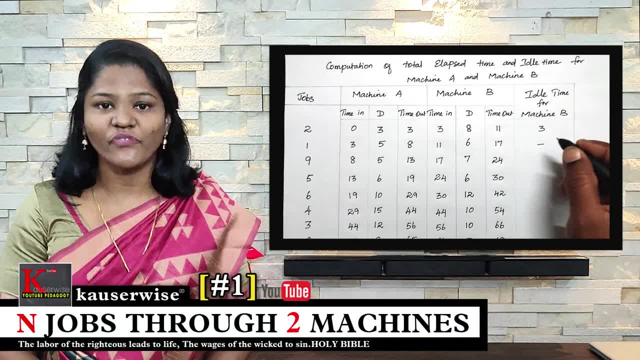 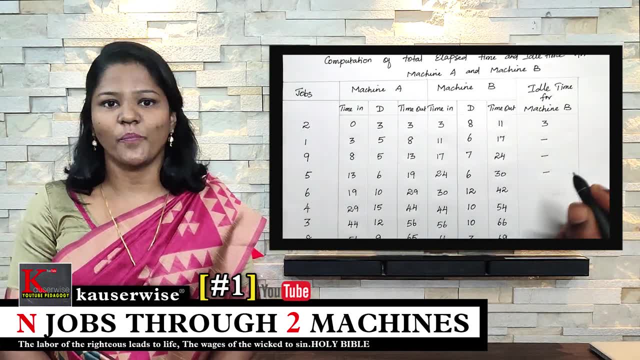 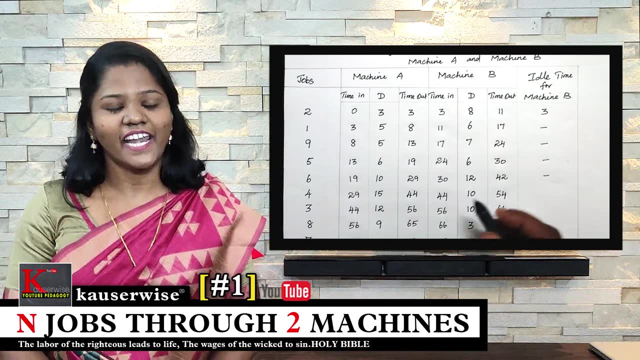 Hi, welcome to Couserwise channel. In this series of videos we are going to see sequential problem, So please try to watch the complete series to get the clarity about this topic. And now in this video we are going to see one numerical problem on n jobs through two machines. Now let's get. 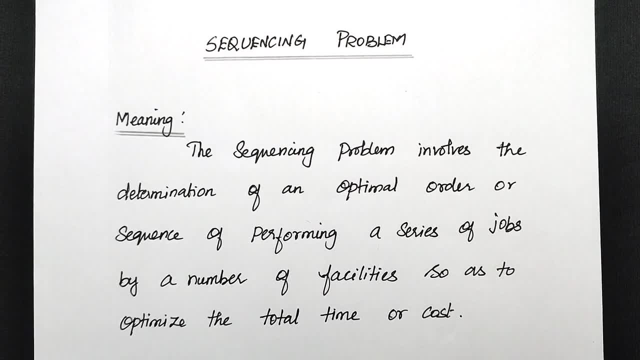 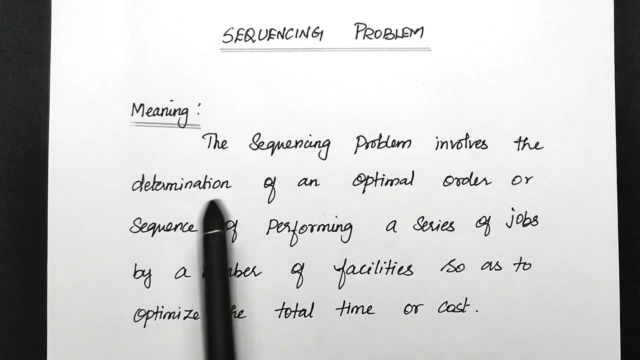 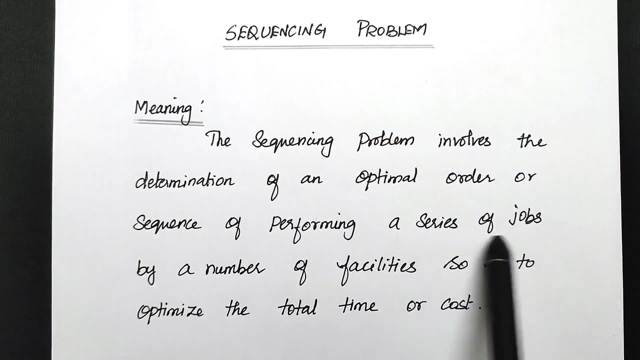 into the video. See before we see the numerical problem, let us try to understand the meaning of sequencing problem. So what is sequencing problem? It involves the determination of an optimal order or optimal sequence of a performing a series of jobs by a number of facilities, so as 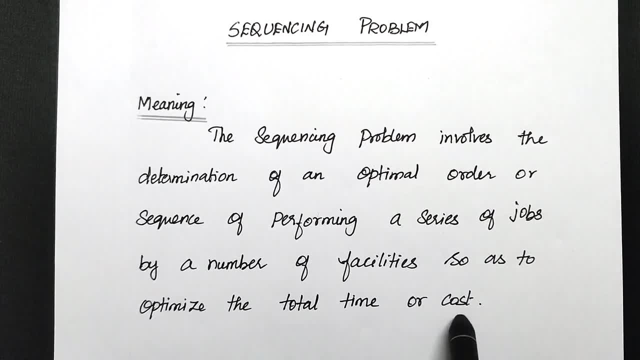 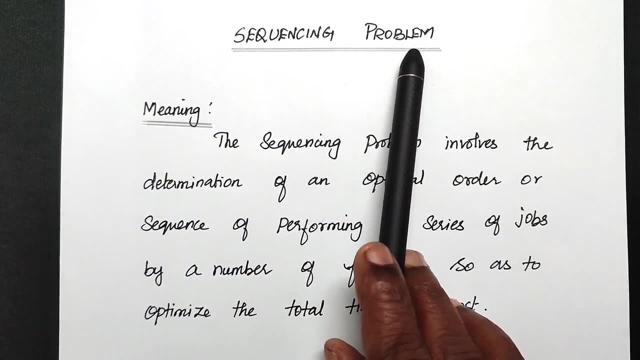 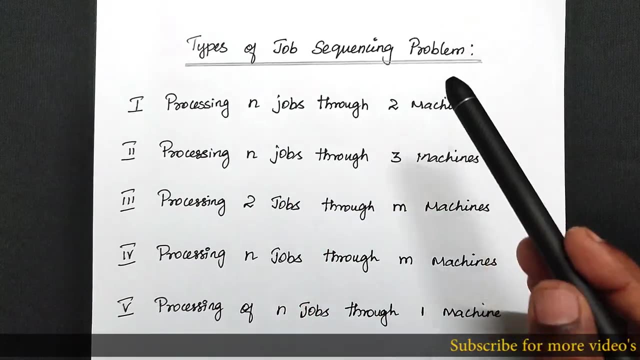 to optimize the total time or optimize the total cost. Here number of facilities means number of machines. So this is the meaning of sequencing problem. Now let us see the different types of sequencing problem. Types of job sequencing problem. Okay, here we have five different types of sequencing problem. 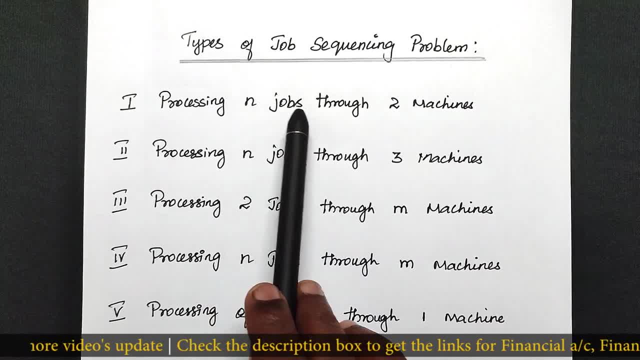 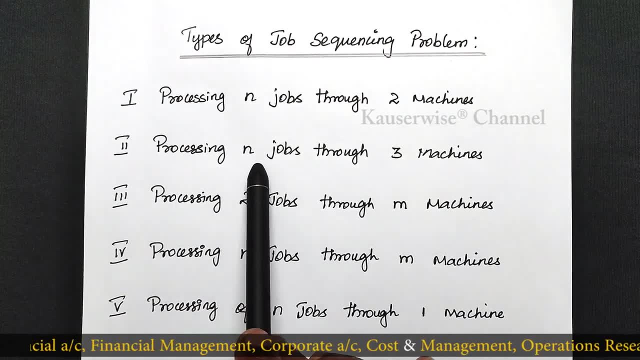 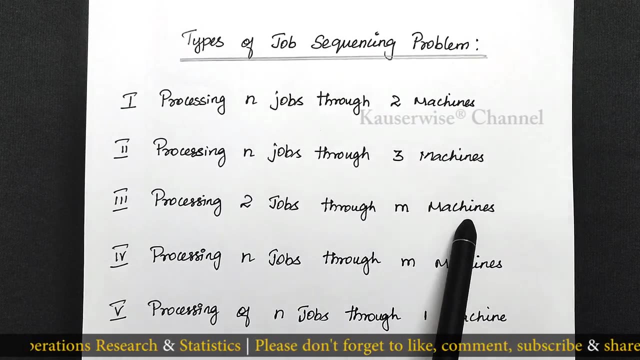 The first one is processing n number of jobs through two machines- Okay. and the next one is processing n jobs through three machines. And the next one processing two jobs through m machines- Okay. and the next one processing n jobs through m machines. 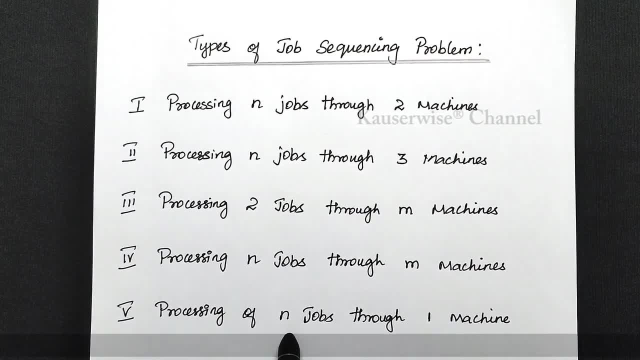 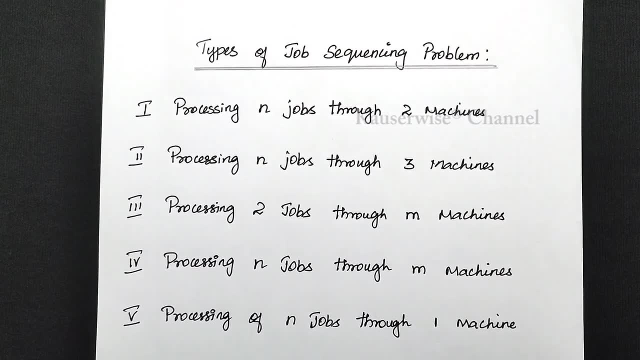 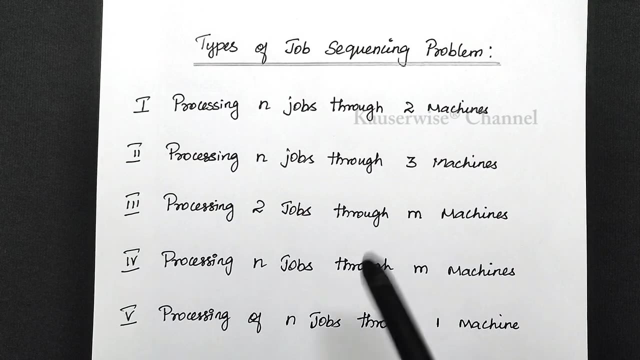 And the last one processing n jobs through one machine. So these are the five different types of sequencing problem. So we are going to see numerical problem for each and every model separately. Okay, now we are going to see the numerical problem for the first one, that is. 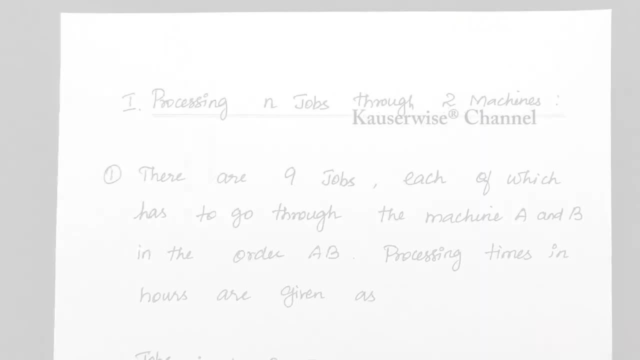 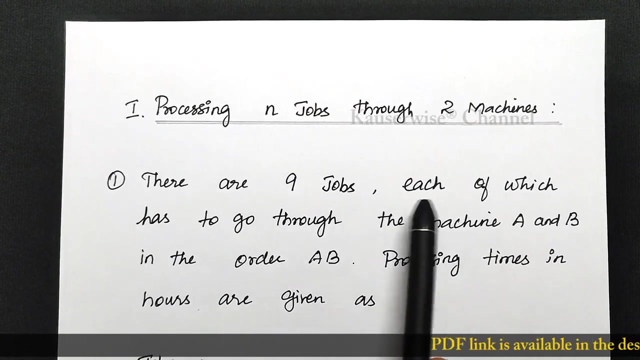 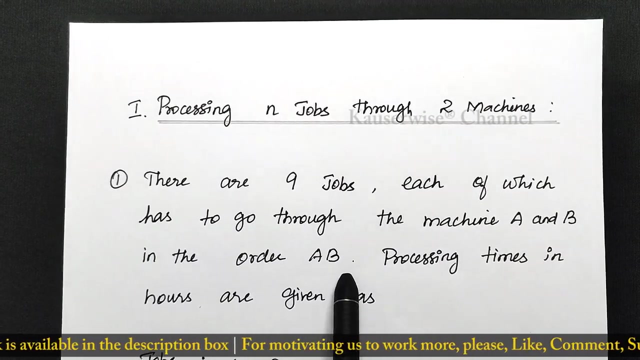 processing n jobs through two machines. See the problem: processing n jobs through two machines. Okay, there are nine jobs, Each of which has to go through the machine A and B. in the order A B. Processing times in hours are given as: 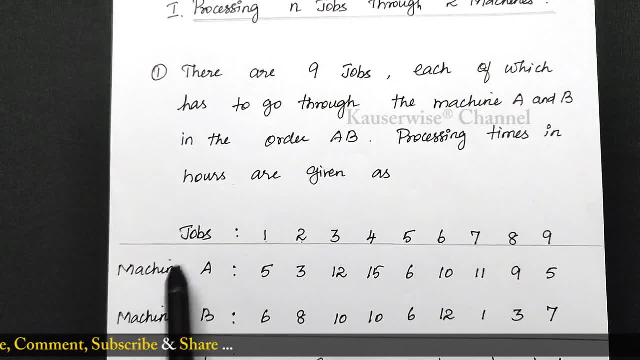 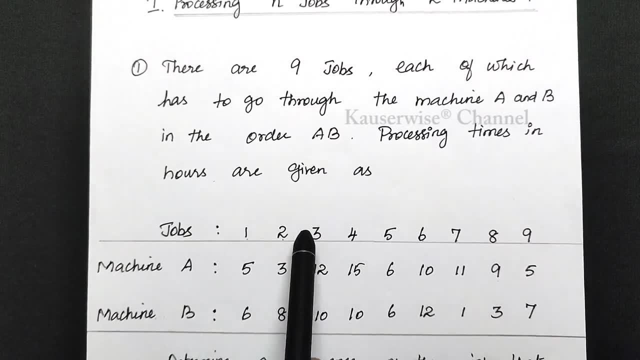 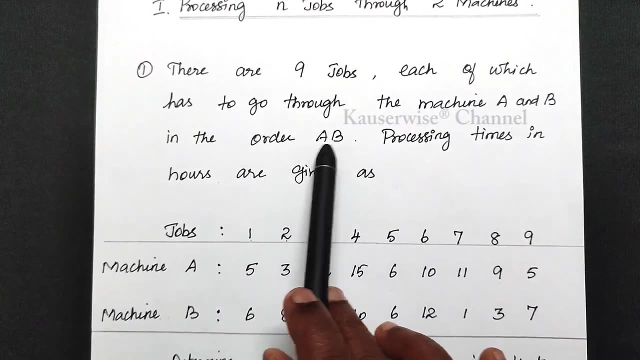 here we have nine jobs, Okay, and here we have two machines, machine A and machine B, And these are the processing time, Okay, so each and every job has to process through machine A first and then machine B. So this is the order. 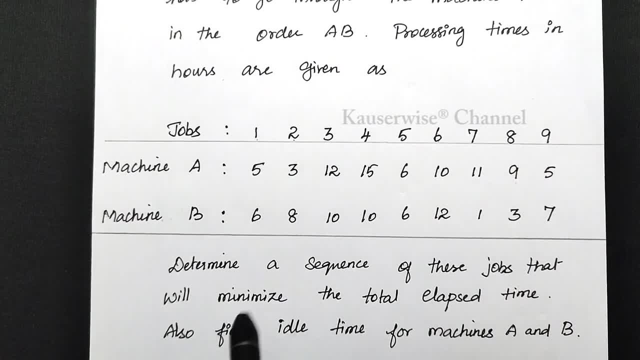 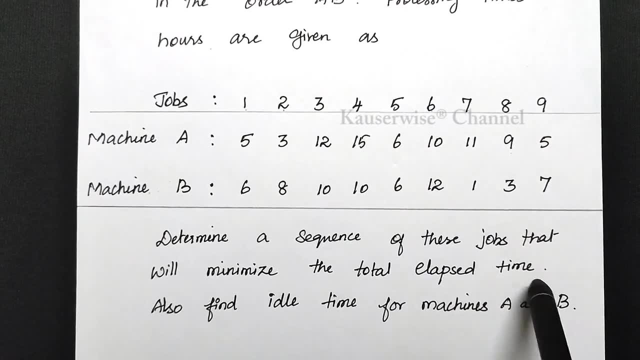 Okay, so each and every job has to process through mission A first and then mission B. So this is the order. Fine, Now, with this information they are asking you to find out, determine a sequence of these jobs that will minimize the total elapsed time. Also, find idle time for mission A and mission B. 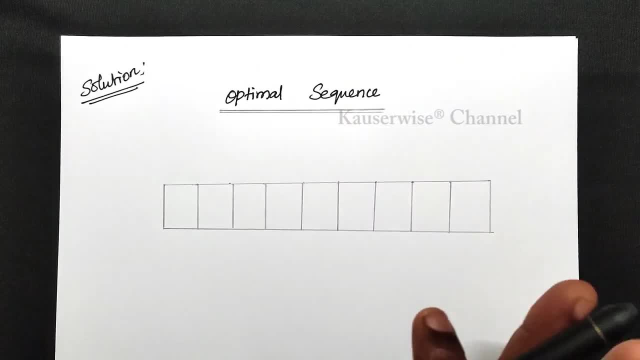 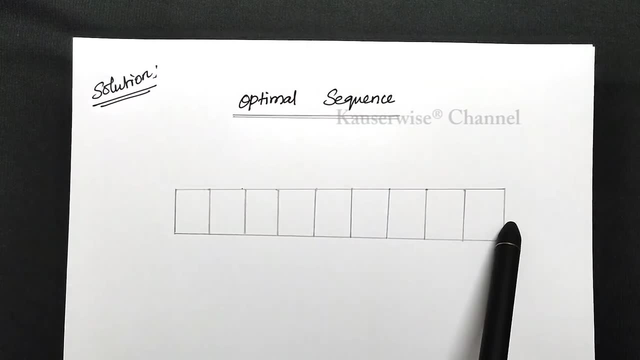 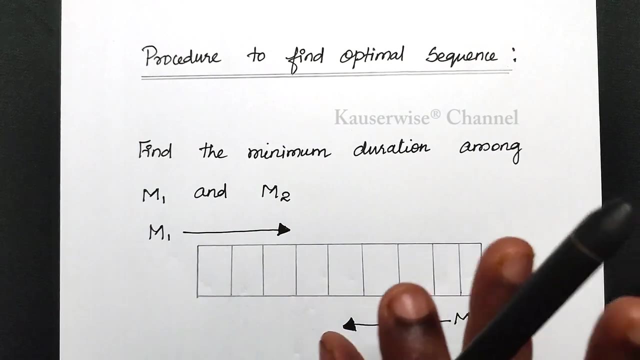 Now we are going to see the solution for this problem. First we need to find out the optimal job sequence. Then we will move to next step. Now look at the simple procedure for finding optimal job sequence. See the procedure to find optimal sequence. First we need to find 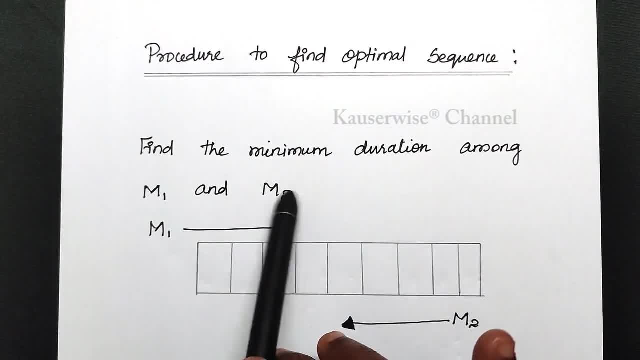 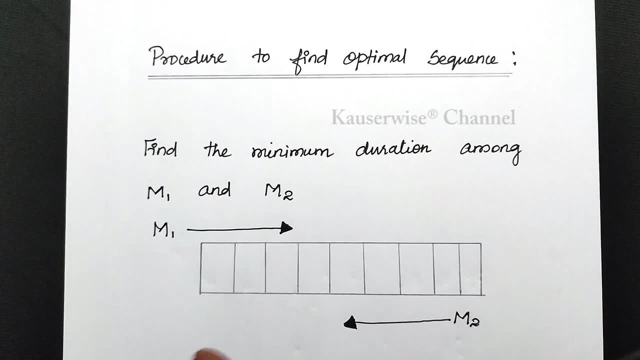 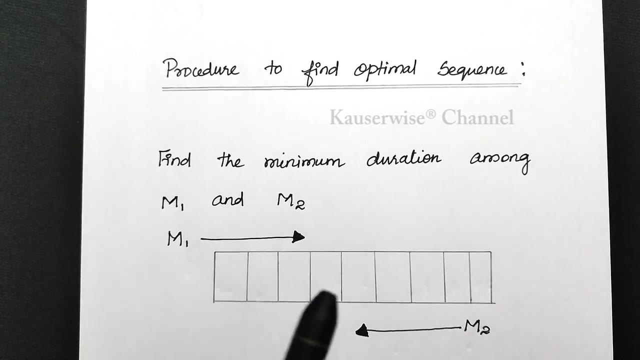 the minimum duration among mission A and mission B. And if you find the minimum duration occurs in mission A, then we need to assign that particular job in the forward direction, first and next, next, like that for mission A And if the minimum duration occurs in mission B. 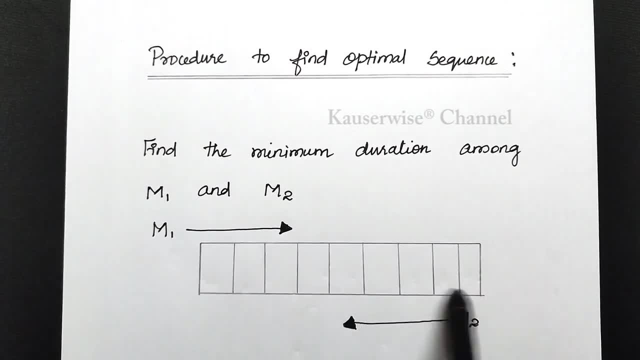 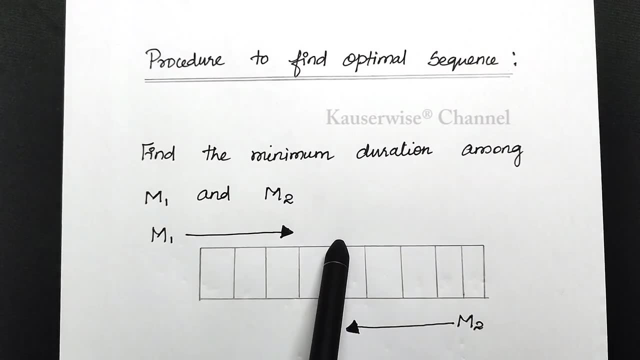 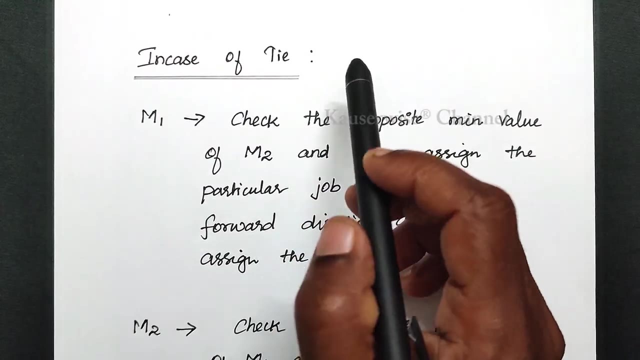 then we need to assign that particular job in the forward direction, In the backward direction first, next, next, like that for mission B. So forward direction is applicable only for mission A and backward direction is only applicable for mission B. Okay, See, the next procedure is in case of tie. See, there are three different situations are. 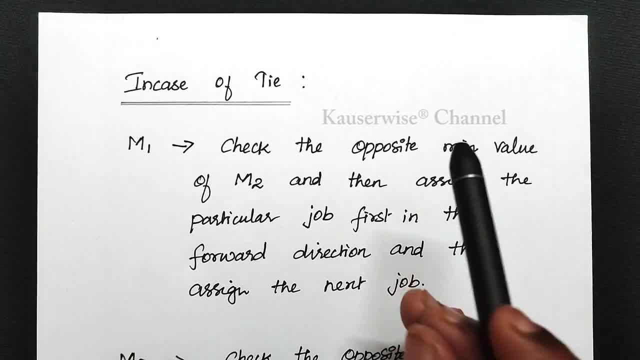 there for tie. that we will see along with the problem for better understanding. Okay, Now look at the problem. See the problem. First we need to find out the minimum duration among mission A and mission B And if the minimum duration occurs in mission B. 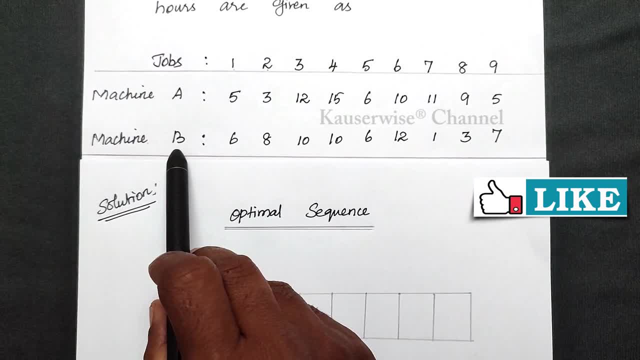 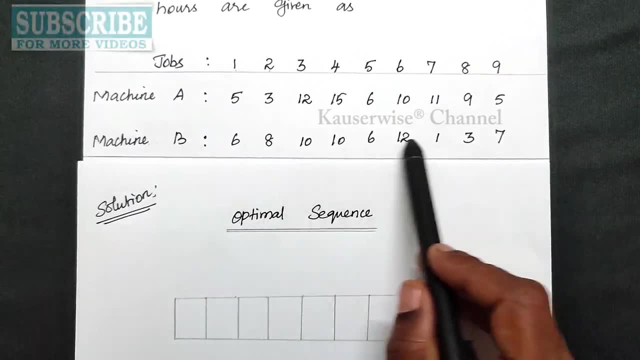 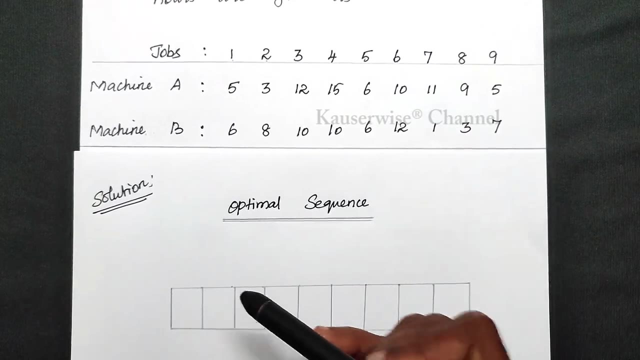 then we need to find out the minimum duration among mission A and mission B, So which one is minimum duration? This is the minimum duration. This occurs on mission B and seventh job. Okay, So this seventh job has to assign in the backward direction. The reason is the minimum duration. 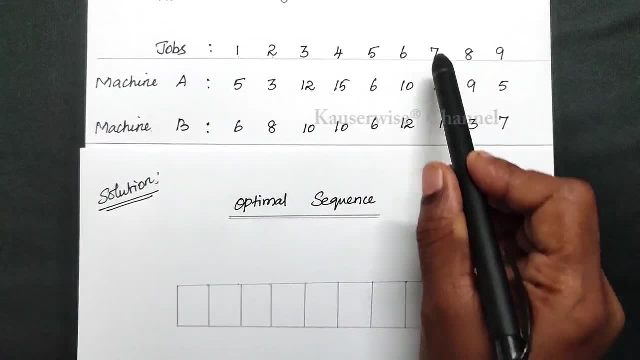 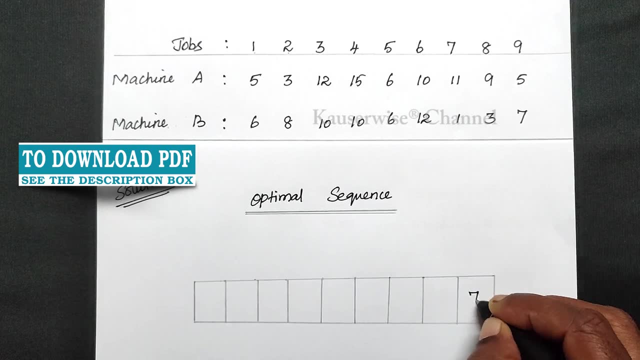 occurs on mission B. So we need to assign this particular job in the backward direction. first, Job number 7, you have to assign Here in this order: Okay, After assigning job 7, again we need to find minimum duration among 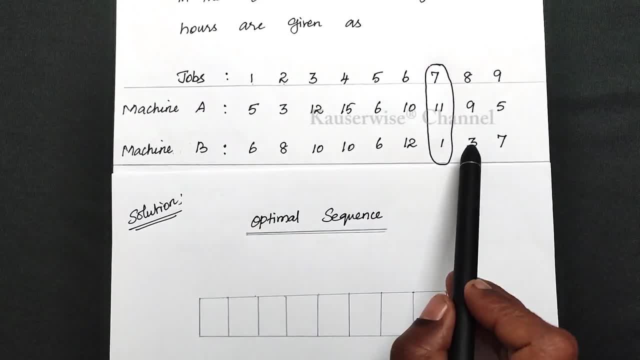 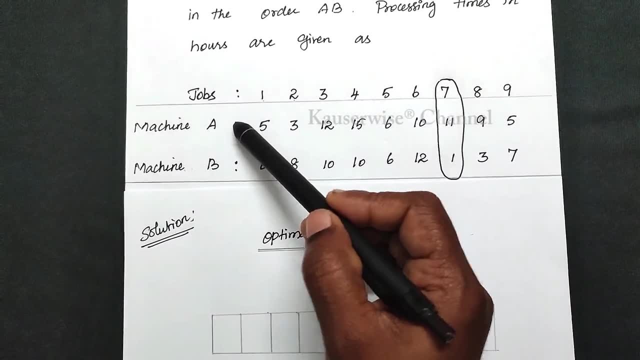 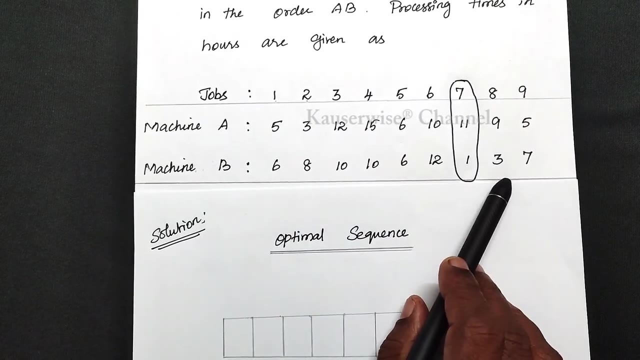 mission A and mission B. Okay, So here 3 is the minimum value, but it occurs in two different places on two different missions: mission A and mission B. Okay, So this is not tie Why? Because it occurs in two different places for different jobs and different missions. So simply you can. 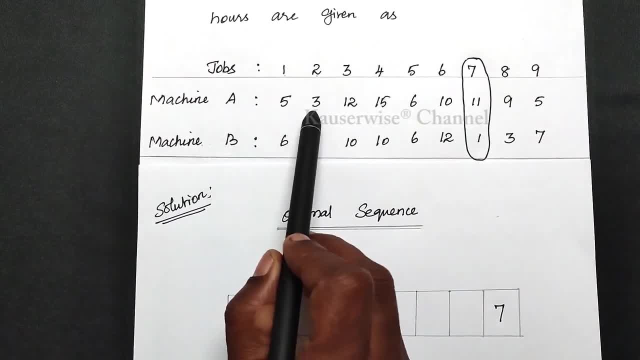 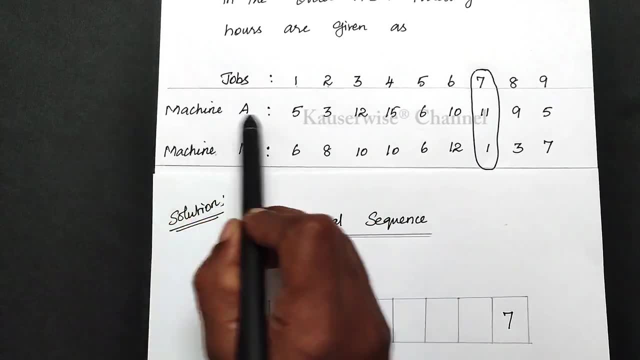 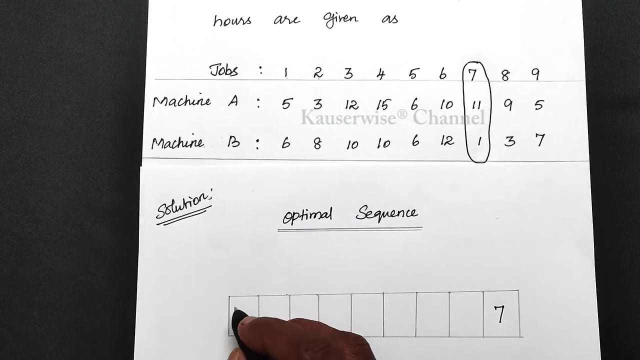 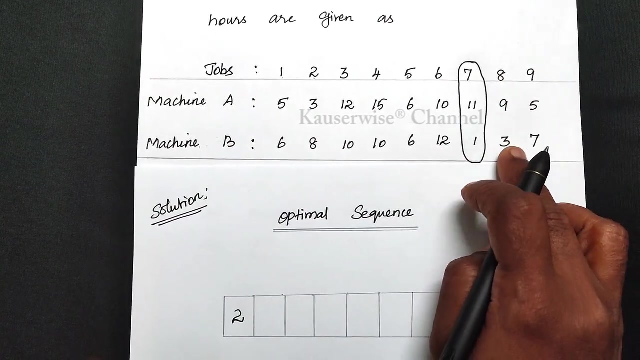 apply the procedure. What is the procedure? For mission A- forward direction. For mission B- backward direction. Okay, So here 3 occurs in mission A for job 2.. Okay, So we can assign this particular job in the forward direction, first, Job 2.. Okay, The next 3 occurs in job 8, mission B For mission B. 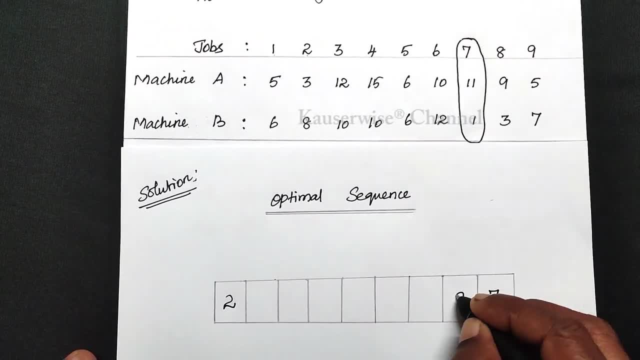 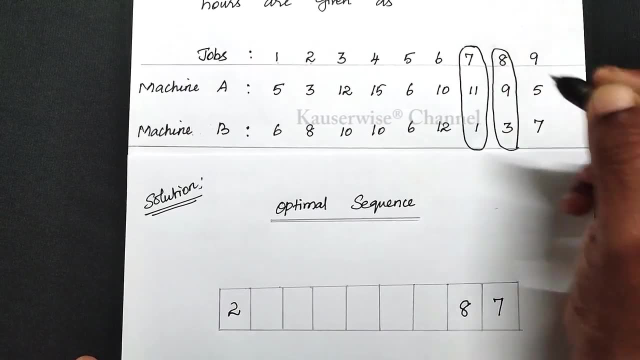 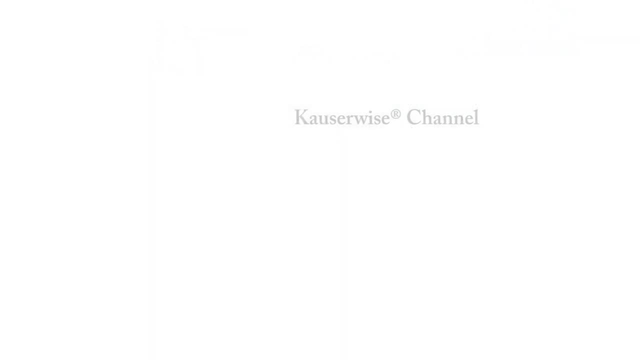 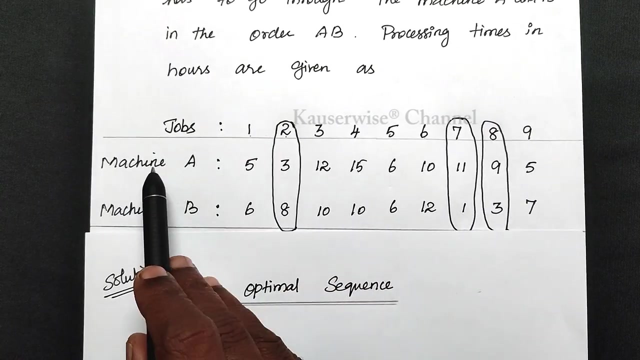 backward direction. No, So assign here Job 8.. Okay, Now you can eliminate the again. we need to follow the same procedure to complete the optimal sequence. See, the next minimum value is 5, but it occurs in two different places, but for same mission, that is, mission A. 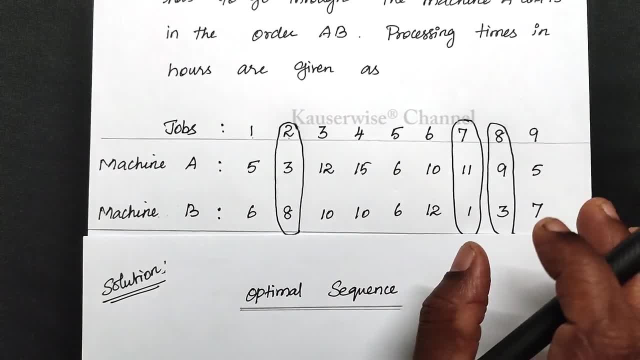 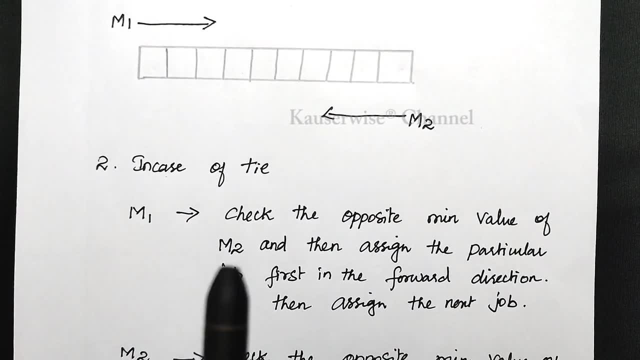 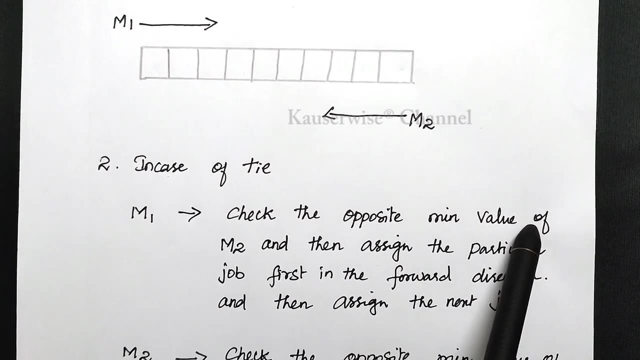 So this is called tie. So there is a procedure in case of tie. Let us see the procedure. See the procedure for in case of tie. Okay, here the tie occurs in machine 1, that is, machine A. okay For that. check the opposite minimum value. 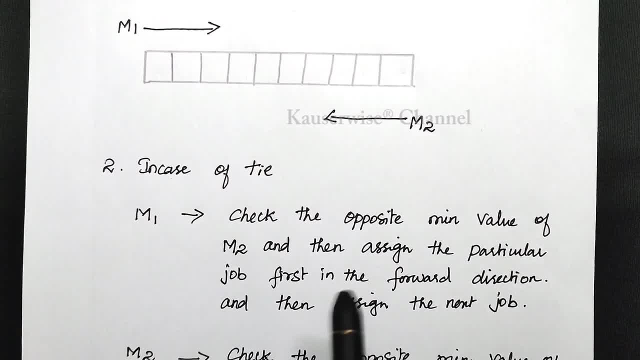 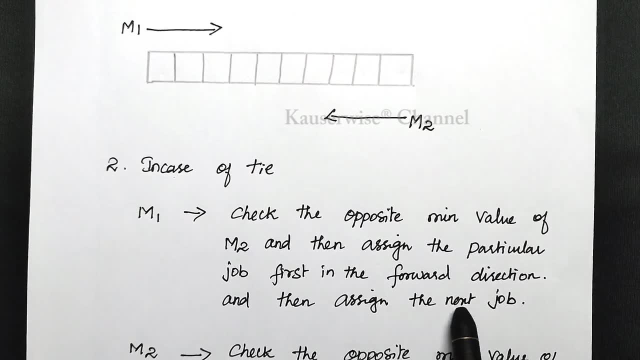 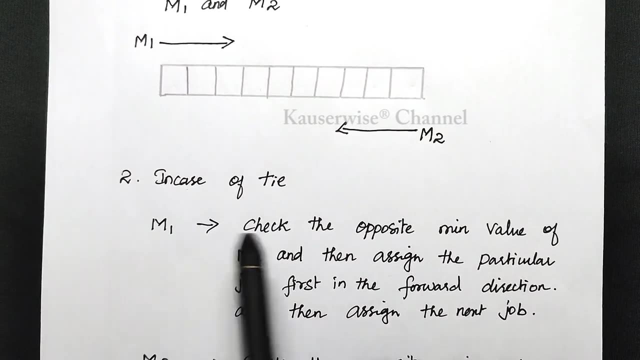 of machine 2, that is machine B in our problem, and then assign the particular job first in the forward direction and then assign the next job. okay, So this is the procedure in case of tie in machine 1.. So we need to find out the minimum value in the opposite machine, that is machine 2.. 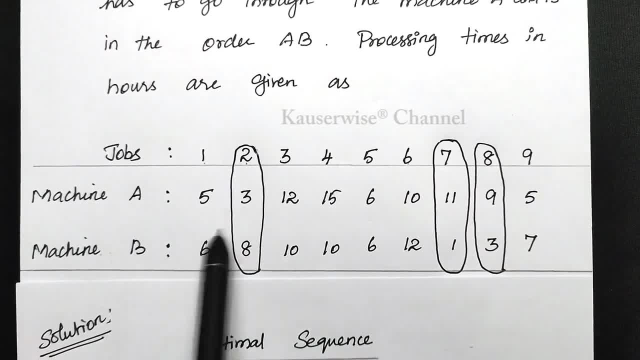 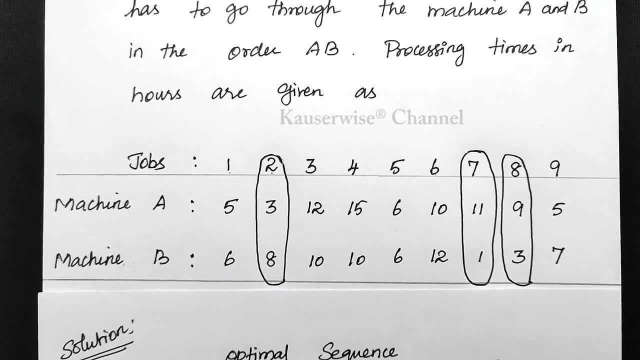 Now see the solution. See the problem Here. the minimum value is 5, no Job 1 as well as job 9, okay, So which job we have to assign first? that is our question, right? So for that we need to. 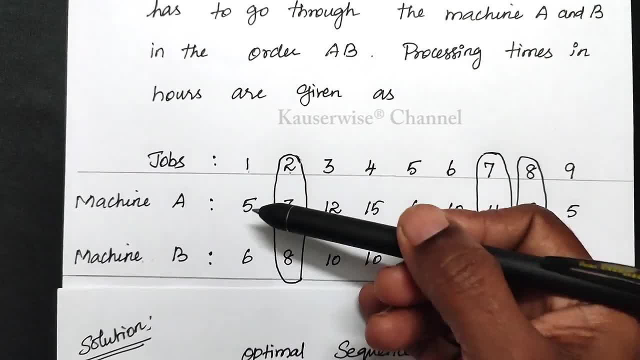 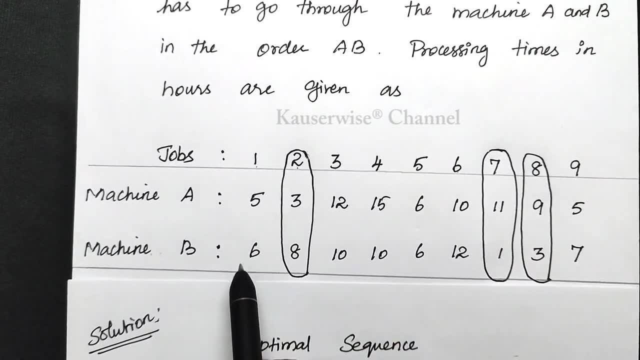 see the opposite value, opposite minimum value. The minimum value will be assigned in the first and the next job will be assigned in the next. okay, So here the opposite value is 6 and here the opposite value is 7.. Which one is minimum, 6 or 7.. 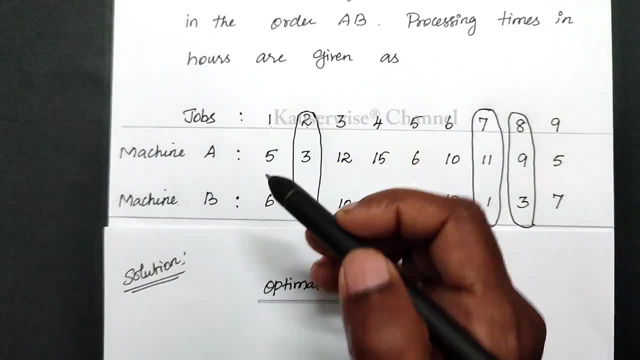 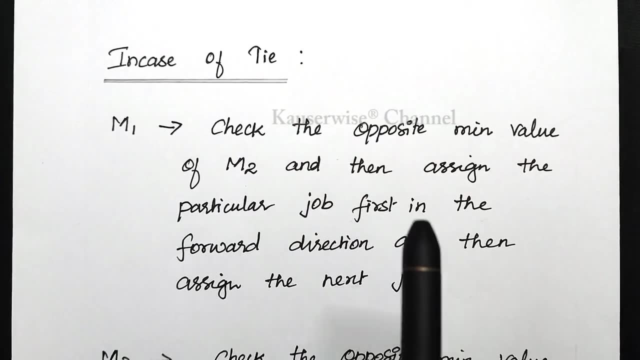 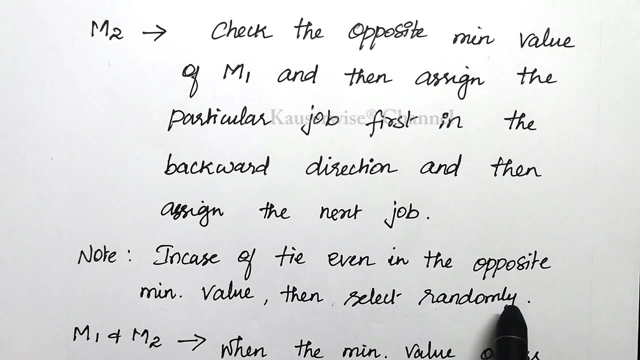 6 is the minimum value, So you can assign job 1 first and then you can assign job 9 next. okay, See one important note: In case of tie, even in the opposite minimum value, then select randomly. that is, we need to select the job randomly and assign them in the forward. 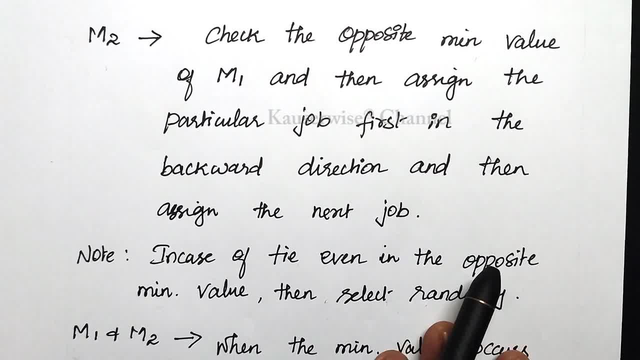 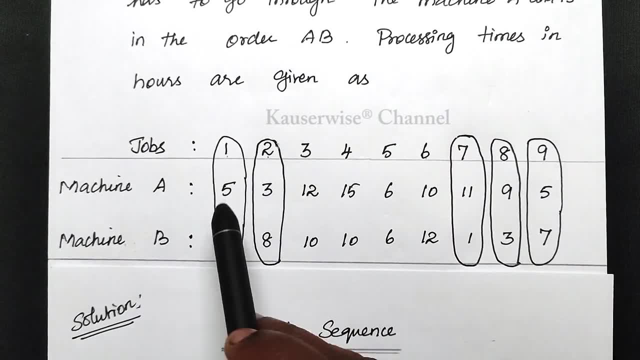 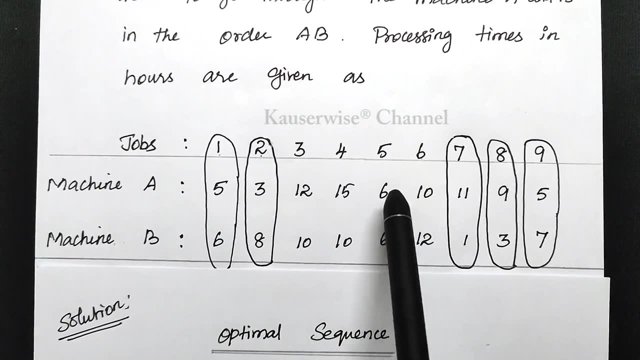 direction for machine A. okay, Now look at the problem. So this is the procedure in case of tie in the first machine. okay, See, we have assigned job 1 and job 9, okay, Again, we need to find out the minimum duration. So which is the minimum duration? 6 is the minimum duration. 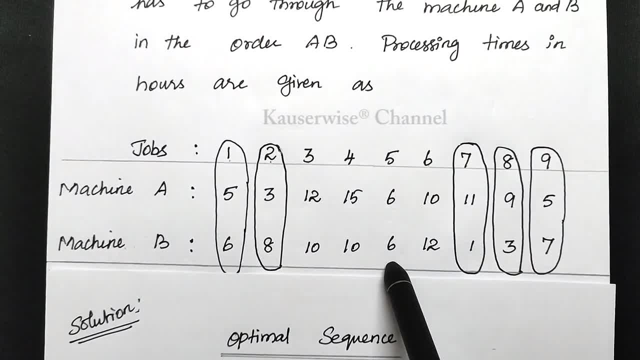 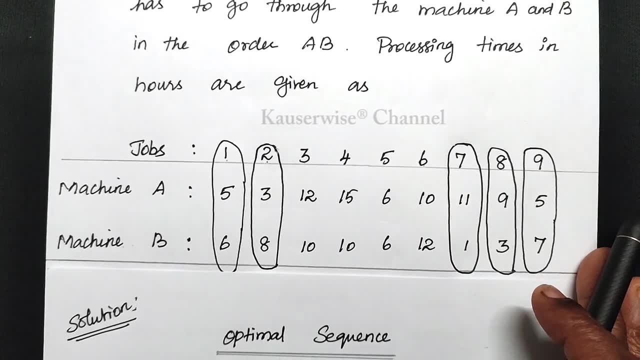 but here it occurs for same job for two different machines, machine A and machine B. okay, This is also one kind of tie. Let us see the procedure. See the procedure when the minimum value occurs in M1 and M2, that is minimum value. So this is the procedure. So this is the procedure, So 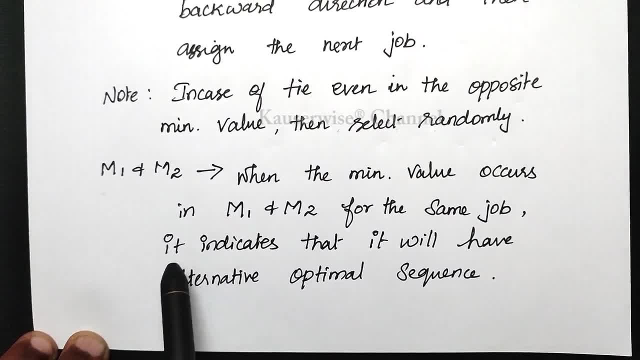 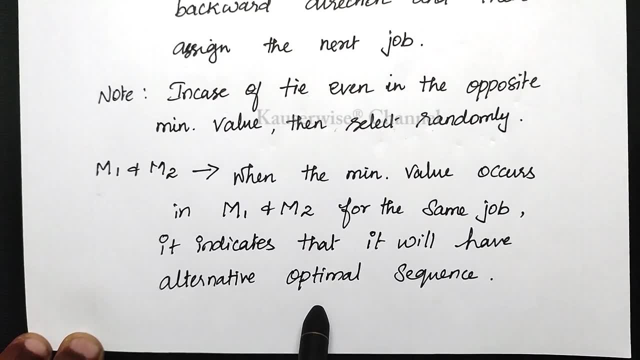 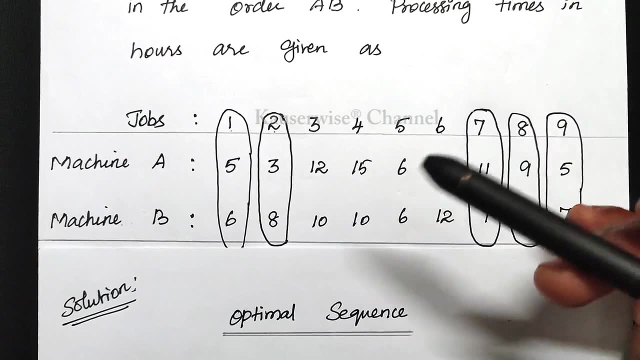 machine A and machine B for the same job. it indicates that it will have alternative optimal sequence. okay, So we will see this point along with the problem for better understanding. Now look at the problem. So here we have two alternative sequence, that is the first. one is: 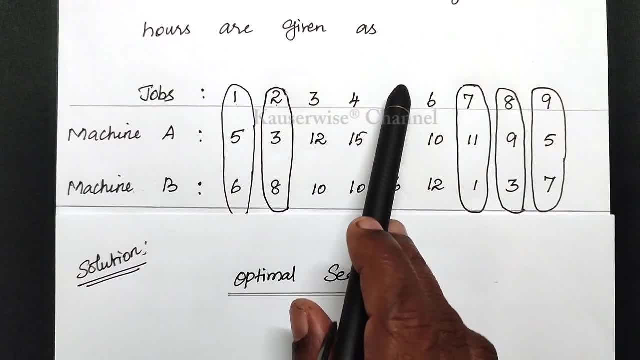 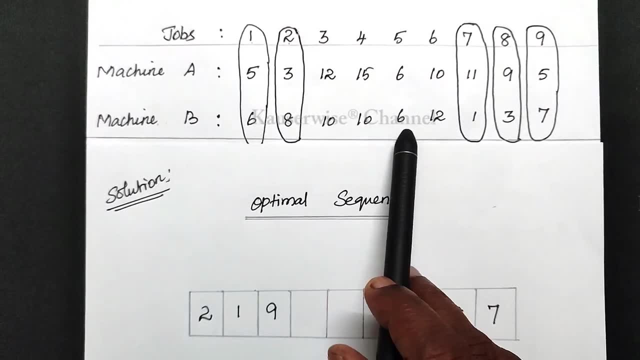 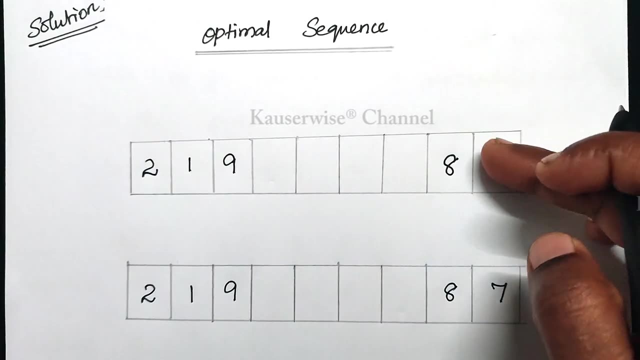 if we consider machine A, we have to assign this job in the forward direction. okay. If we consider this 6- that is, machine B- we need to assign job 1 and job 9 in the forward direction. okay, So we need to assign job 5 in the backward direction. See, this kind of tie will have two alternative. 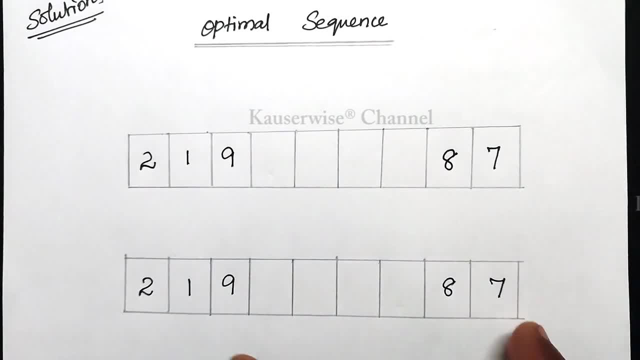 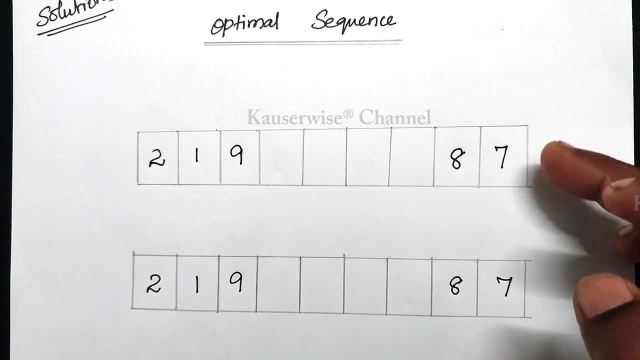 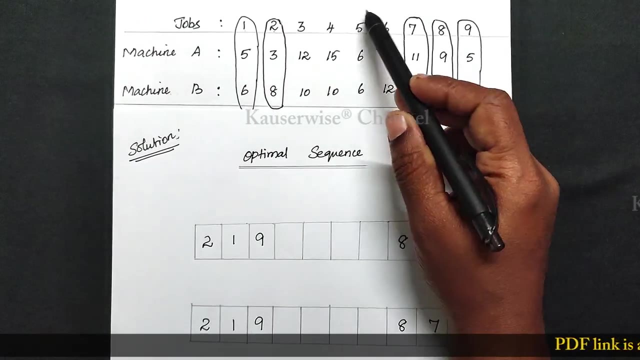 optimal sequence. Just copy the same sequence. Now we are going to decide that particular job, whether to assign in the forward direction or backward direction, but for both- optimal sequence. we are going to get the same answer. See the problem for this particular job, that is, job 5. 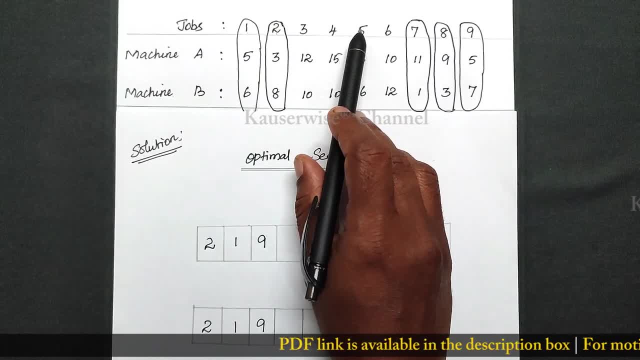 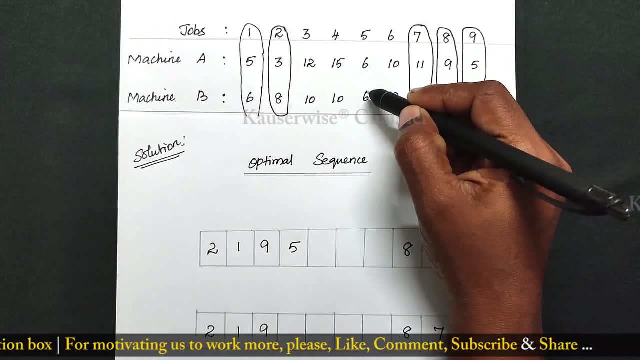 if we consider machine A, we have to assign job 5 in the forward direction. okay, So we need to assign job 5 in the forward direction. okay, Job 5 will be assigned here. If we consider machine B, then we have to assign this particular job in the backward direction. So assign 5 here. So 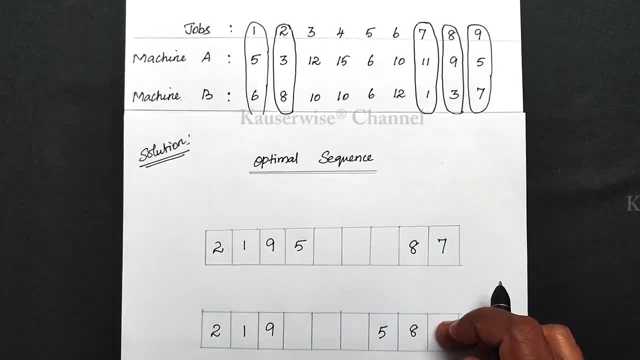 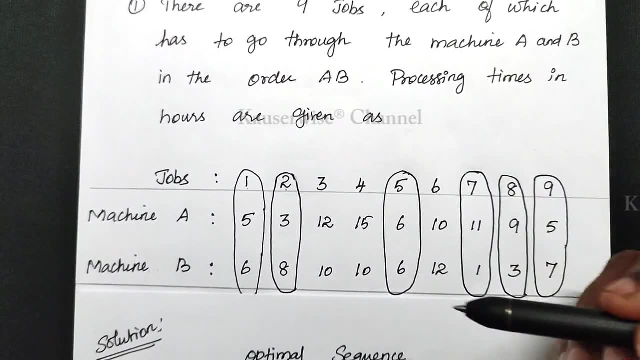 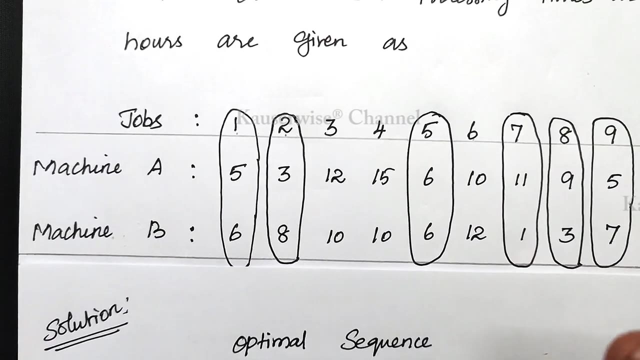 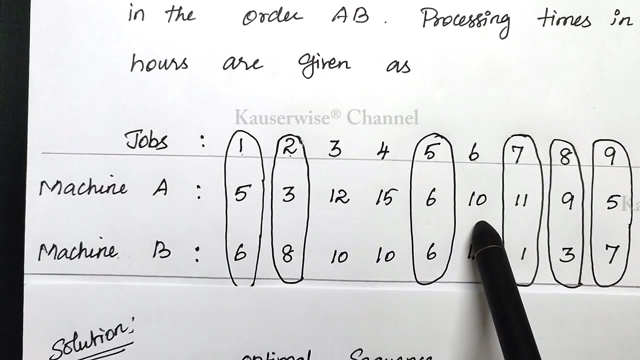 here we have two different alternative optimal sequence. okay, See, after assigning job 5 in two alternative optimal sequence table, again you have to find out the minimum value. See here the minimum value is 10 but it occurs in three different places. For machine A there is no tie because it occurs in only one particular job. okay, So we can use. 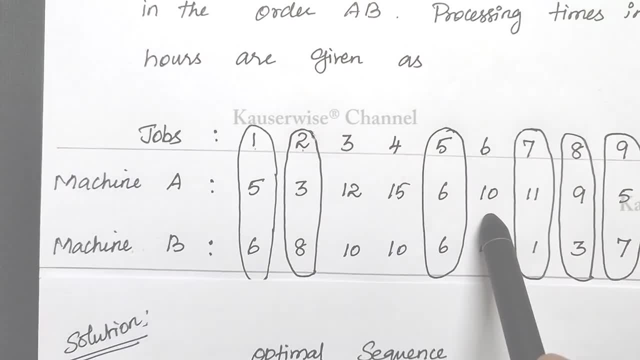 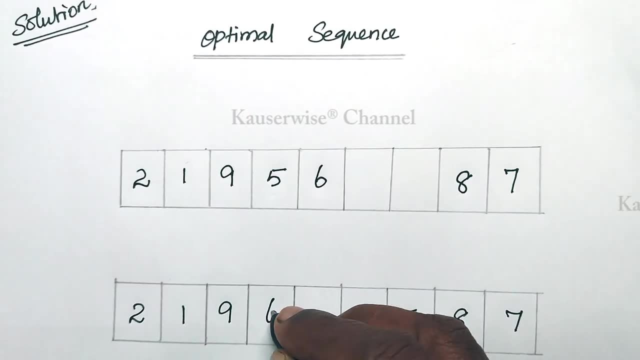 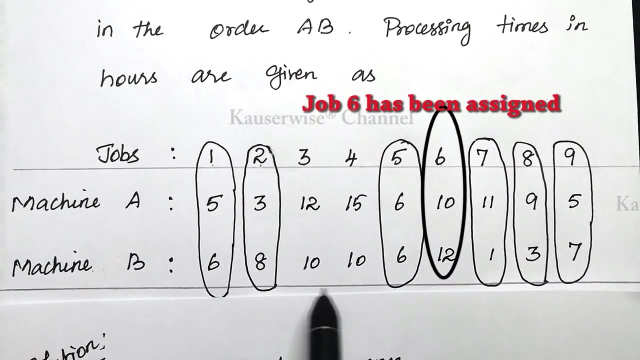 the forward direction and we can assign job 6.. Assign 6 in the forward direction for two different alternative solution: okay, And for the next one, for machine B, there is a tie, because here 10 occurs in two different jobs for the same machine. 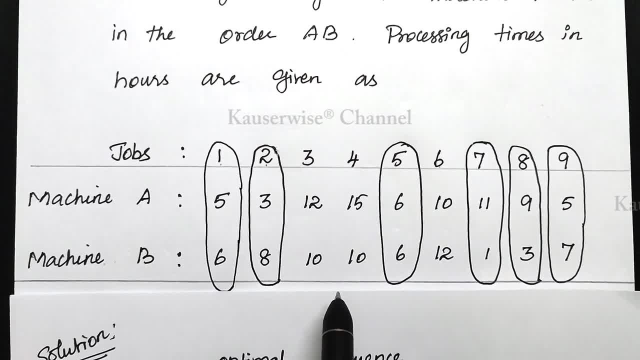 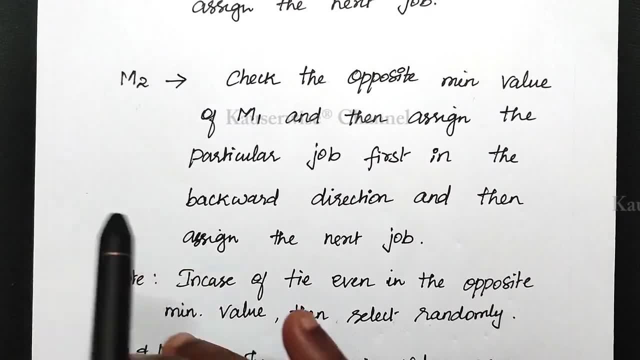 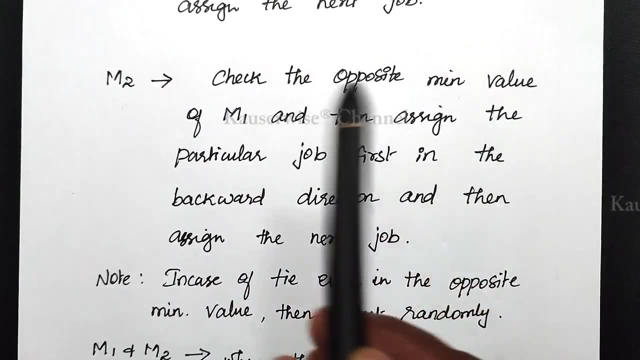 So this is called tie. What is the procedure for tie for the same machine? Look at the procedure for in case of tie on machine B, that is, machine 2.. See, if the machine B has same minimum value, then we need to check the opposite minimum value of machine 1, okay, And then assign the particular. 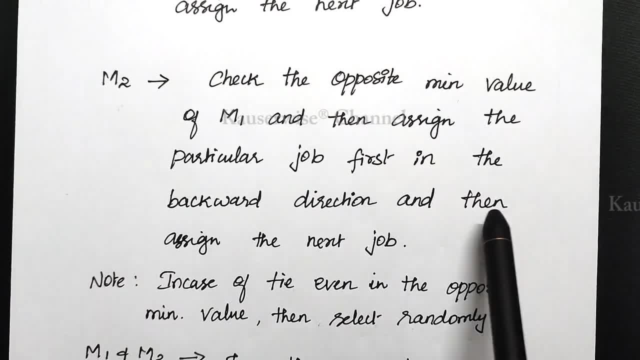 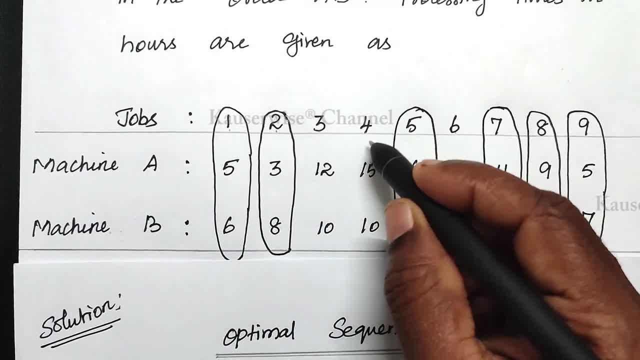 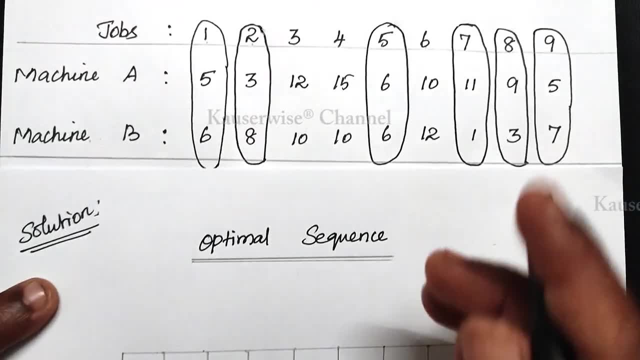 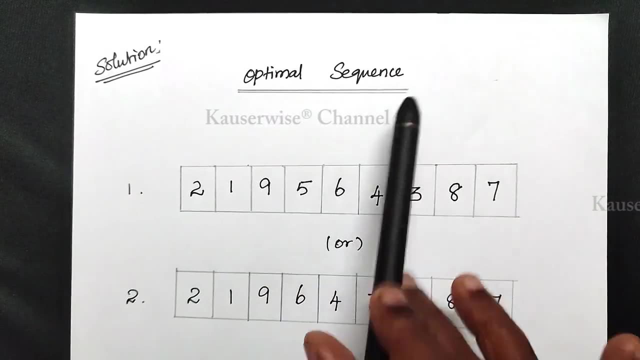 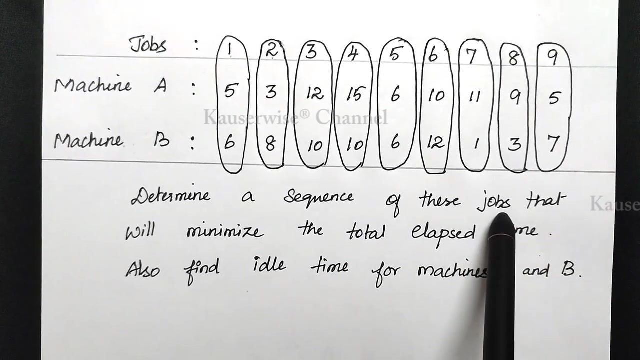 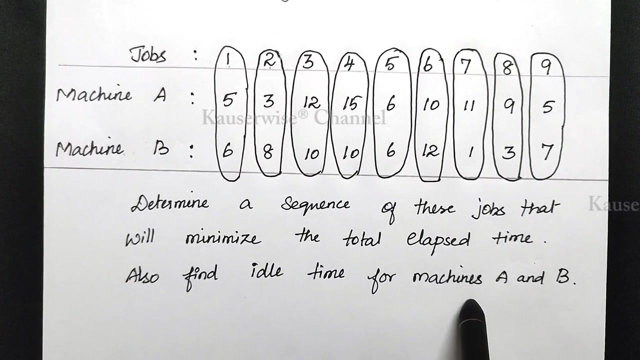 tie. What is the procedure for tie for gold, So this is called tie. What is the procedure for tie for the same machine? So this is called tie. What is the procedure for tie for time for machine A and machine B? okay, The first thing is they are asking us to find out. 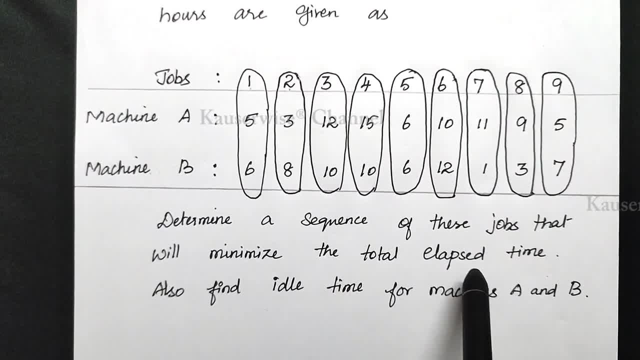 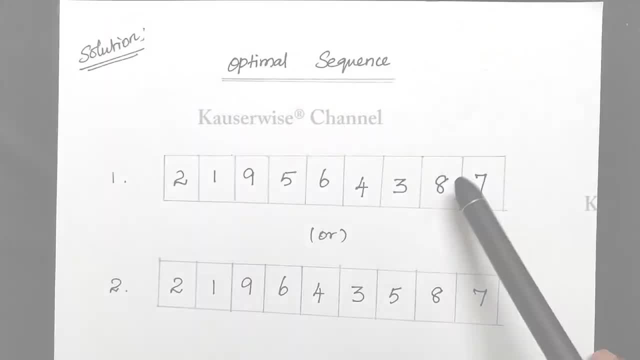 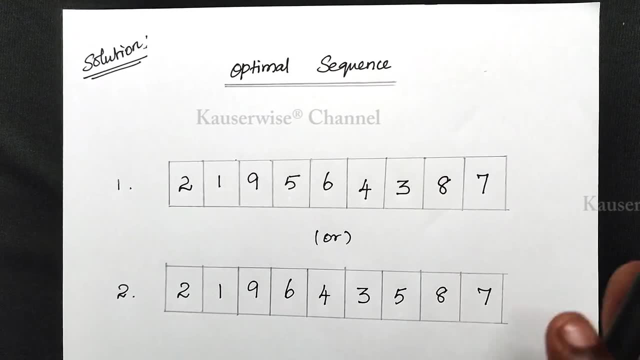 optimum sequence in order to minimize the lapse time and to find out the idle time for machine A and machine B. okay, Now see the solution. See the optimal sequence In this problem. we have got two alternative optimum sequence. okay, Anyway, we are going to get the same answer. 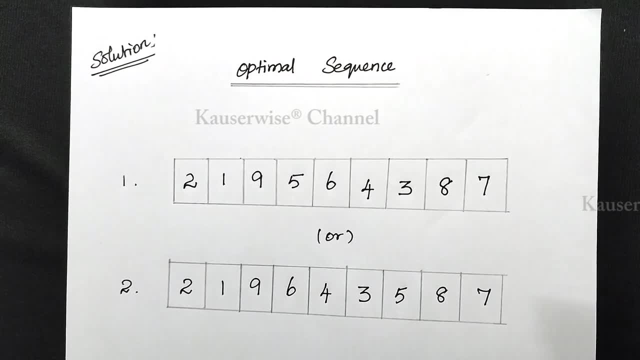 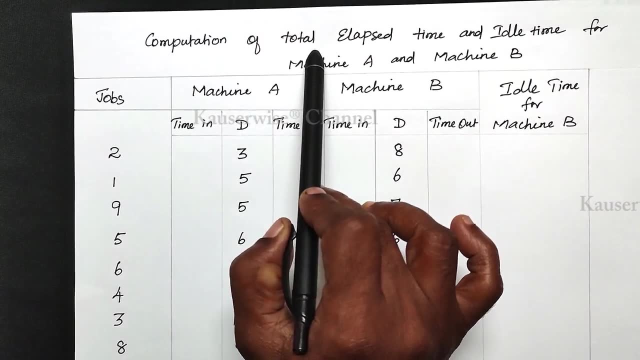 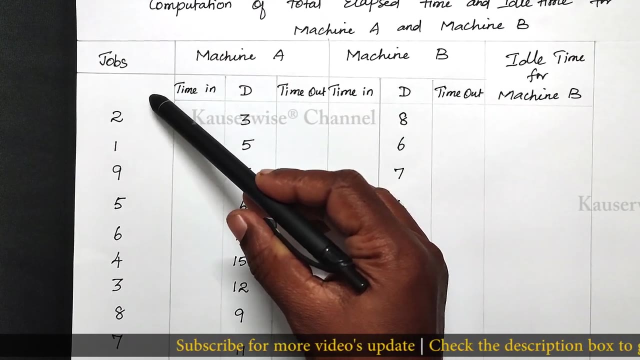 if we proceed with the first one or second one, I am going to take the first one for the further calculation. Let us see the calculation. See the next calculation: computation of total lapse time and idle time for machine A and machine B. okay, And this is the job, based on the optimum. 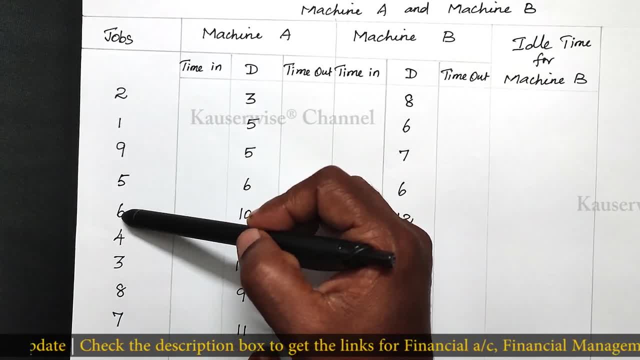 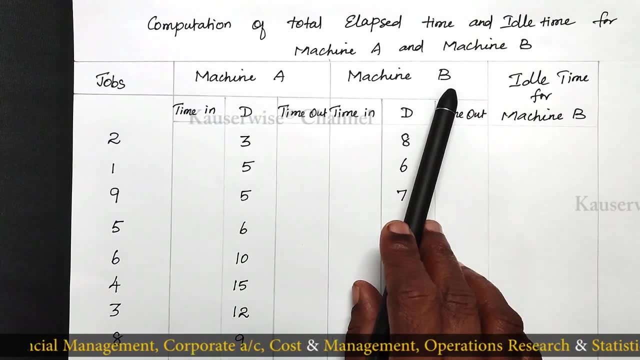 sequence, that is, 2, 1,, 9,, 5,, 6,, 4,, 3,, 8,, 7,. okay, And this is the information for machine A and machine B, that is in time out time and duration, And the next one in time. 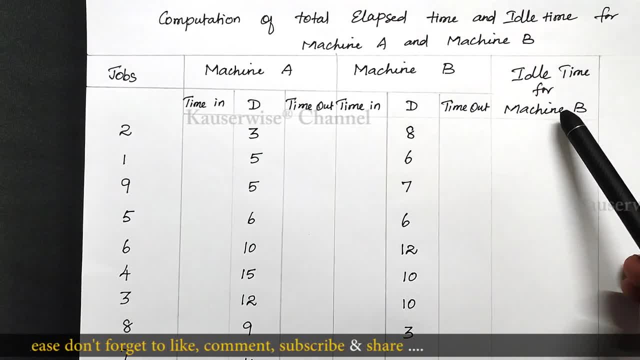 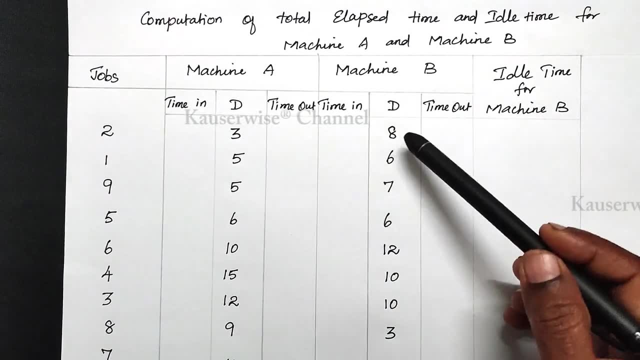 out time and duration. Now let us see the last one. The next one is theě, The next one is the time duration and the last one idle time for machine B. First we need to write the duration for machine A and machine B based on the optimum sequence. Now look at the problem. See the 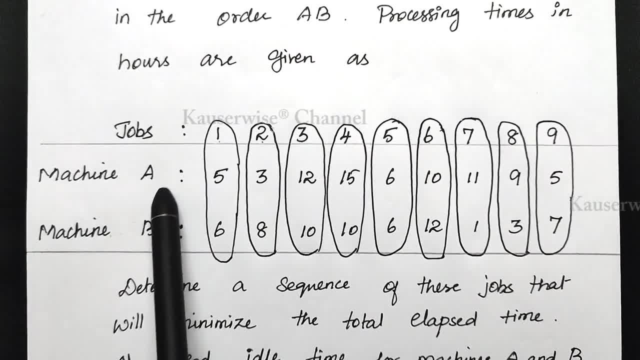 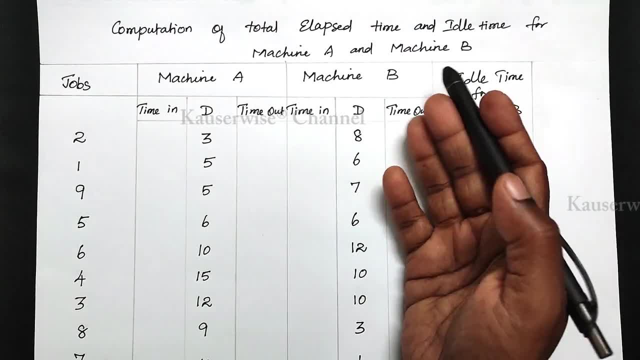 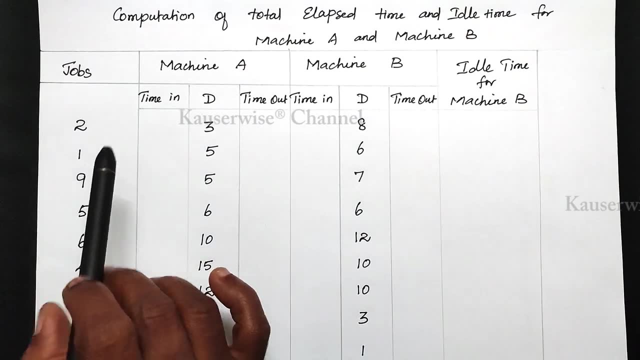 problem. This is the duration for machine A and machine B for 9 different jobs. Now write the duration in the tabular column. Look at the solution. We have written duration for machine A and machine B from the given problem. Now we are going to find out in time and out time for. 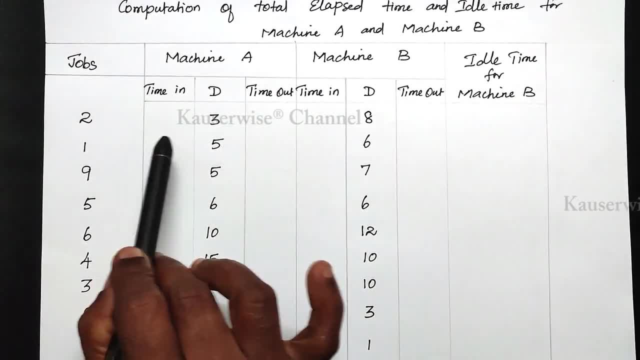 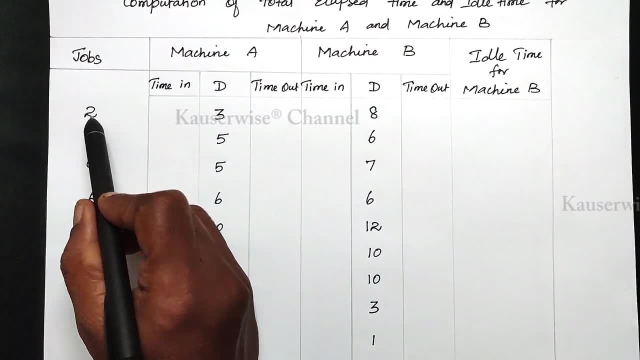 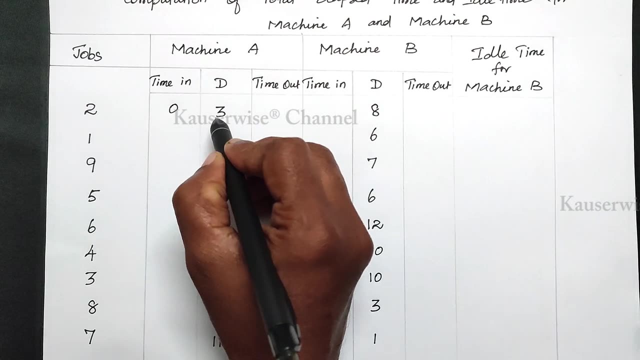 machine A first because there is no idle time for machine A during the process. So first one is job 2.. This is the first job, So in time is 0.. So how to find out out time? Starting time plus duration is equal to out time, So time in is 0.. 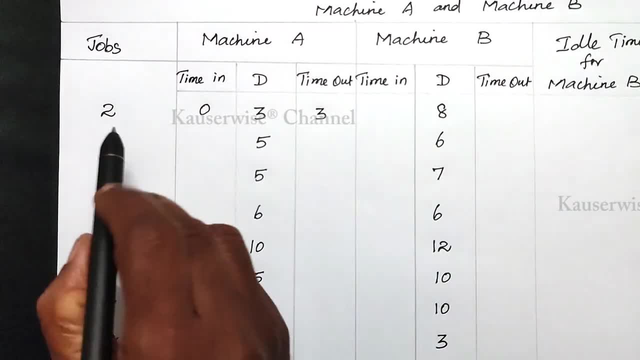 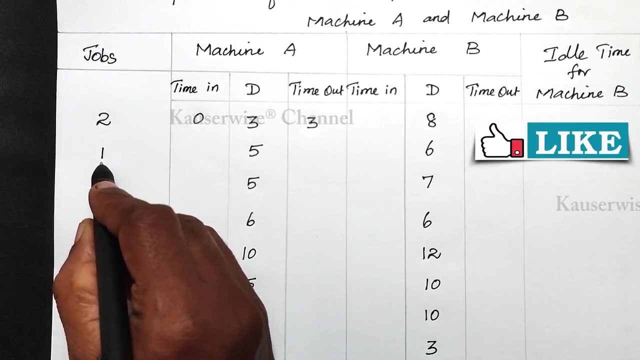 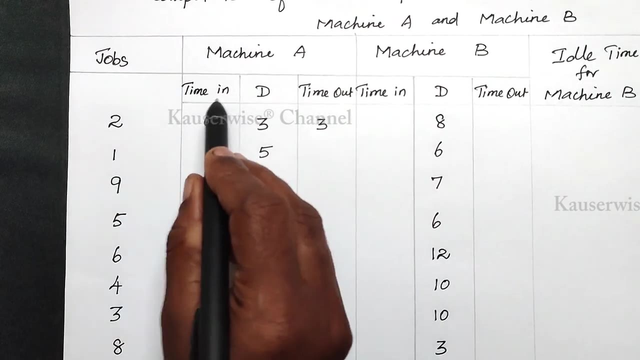 So after processing the job 2, then the machine A will take the second job. The next job is job 1.. What is the in time? So, after completion of the previous job? So after that the machine will take up the next job. So in time for the next job is 3.. The finishing time of the previous job. So 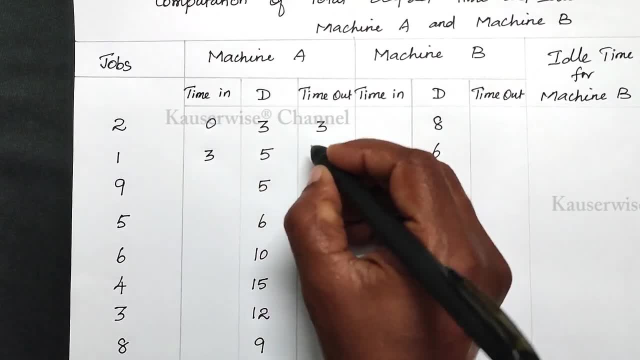 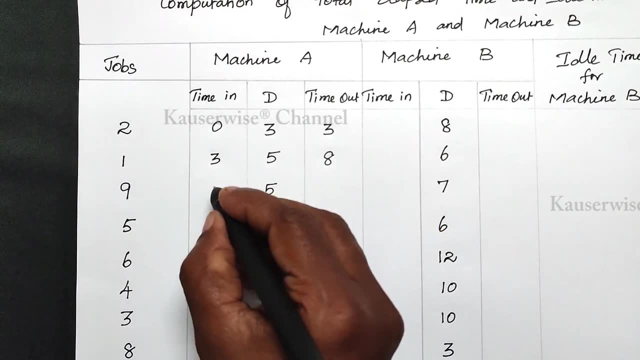 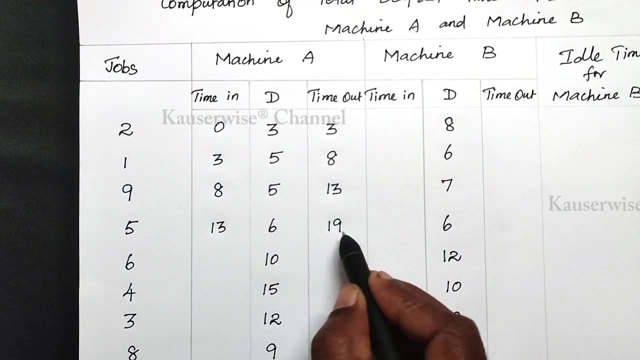 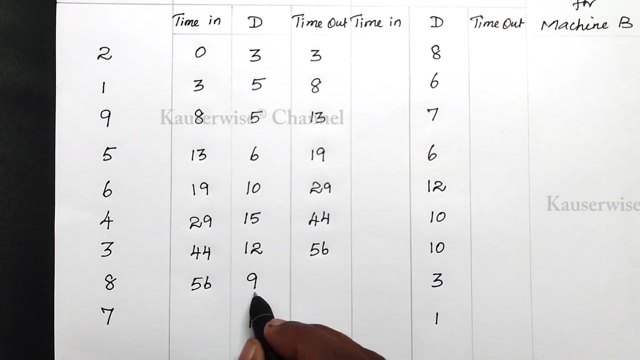 3 plus duration, 5.. 3 plus 5.. Out time is 8.. And then mission A will take up the next job. So in time is 8,, 8 plus 5,, 13 is the out time. Then in time is: 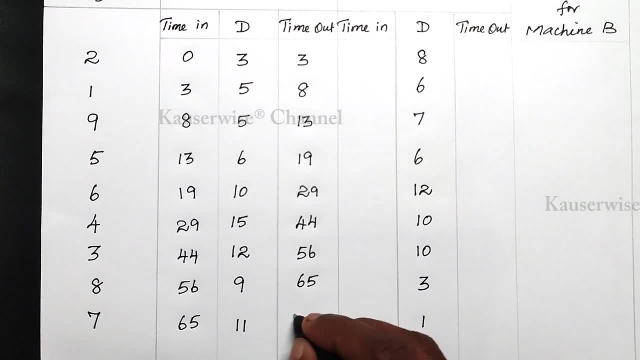 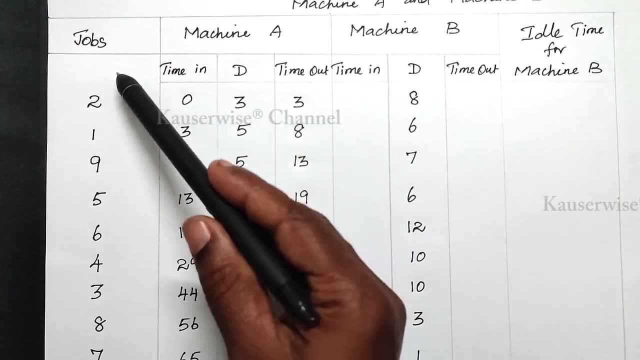 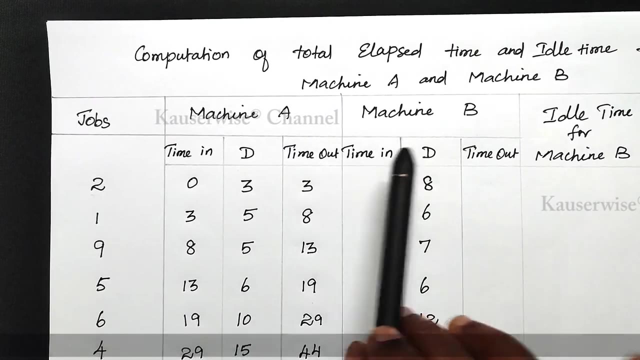 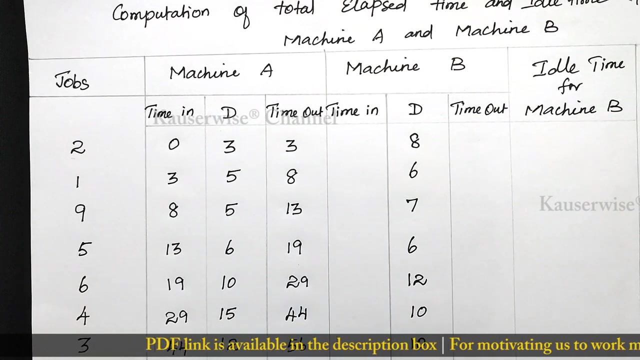 65 plus 11, 76.. This is the way to find out in time and out time for machine A, according to this sequence. Now let us see the calculation for machine B. Now we are going to find out in time and out time for machine B. okay, So here machine A processed 9 different jobs continuously. 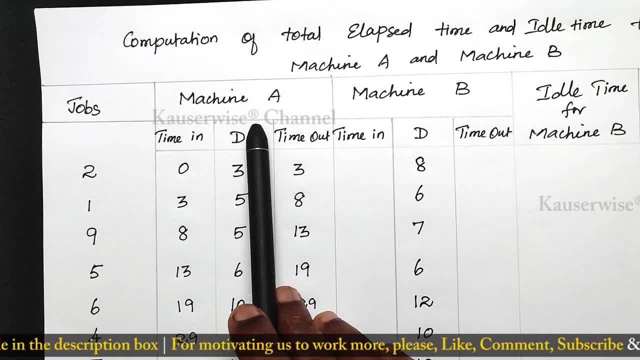 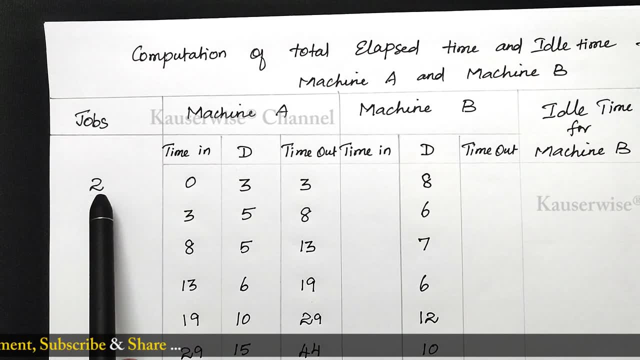 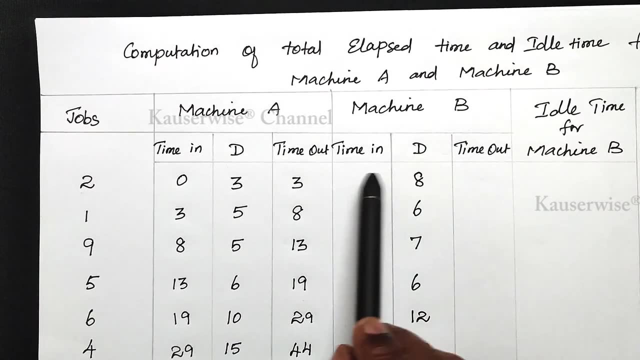 but each and every job should process through machine A and machine B. okay, This is the order. So look at the first job. okay, So job 2 processed through machine A on third hour. Now this is the in time for machine B, for the first job. So 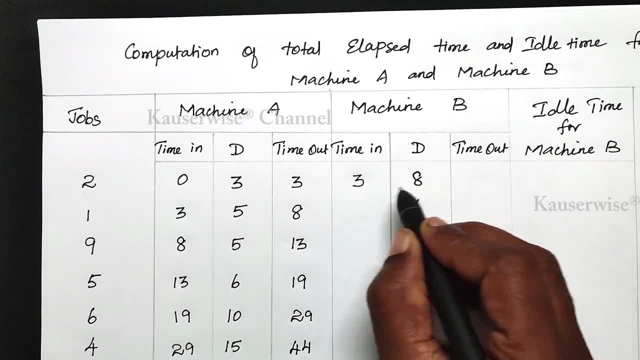 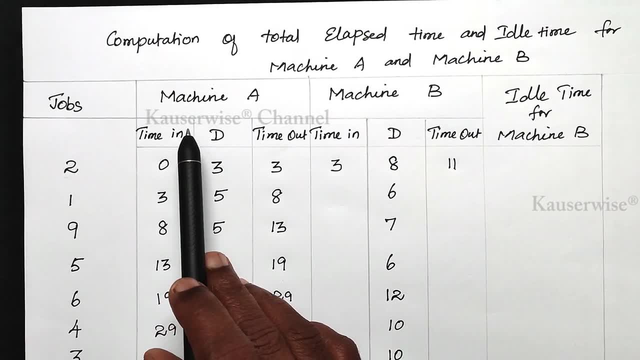 in time is 3 plus duration, 8,, 3 plus 8, you will be getting 11 as out time for the first job. So job 2 has processed through machine A and machine B and completed its process on 11th. 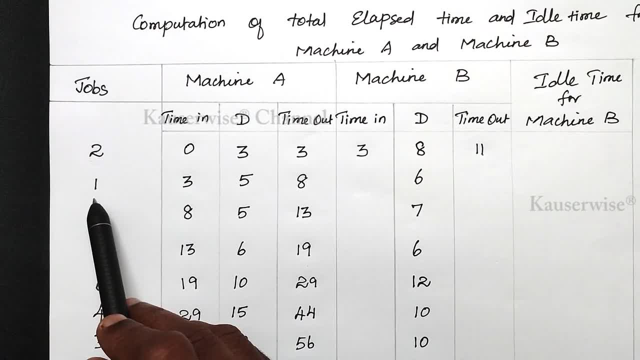 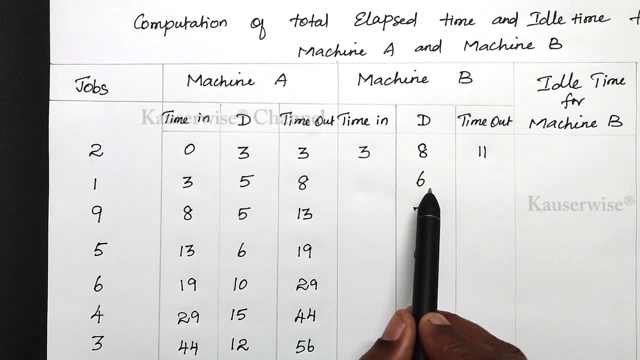 hour. Now look at the next job, job 1. Its out time from machine A is 8th hour only. okay, So this particular job will move on to machine B at 11th hour only. Why? Because machine B will complete. 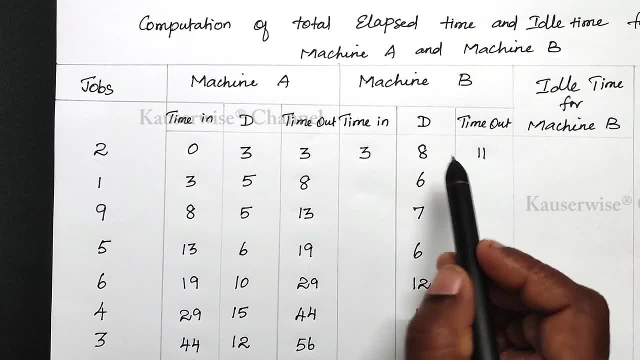 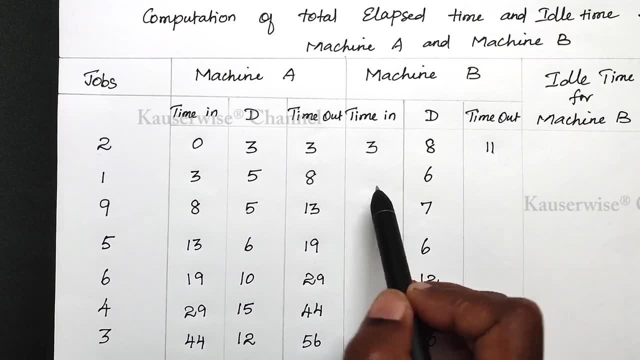 the previous job on 11th hour. So after completing the previous job only it will take up the next job. So machine B will take up the next job on 11th hour. So in time for the next job is 11th. 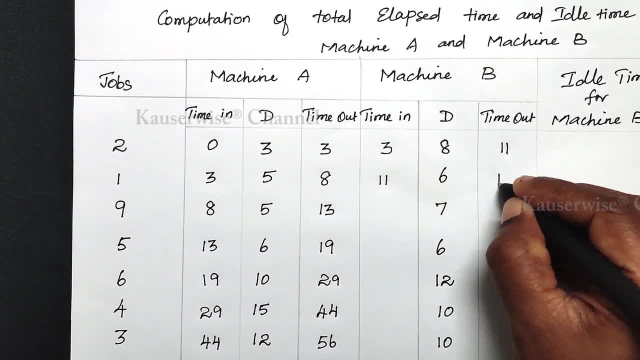 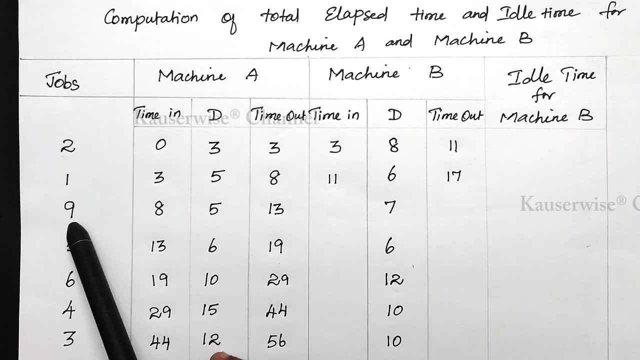 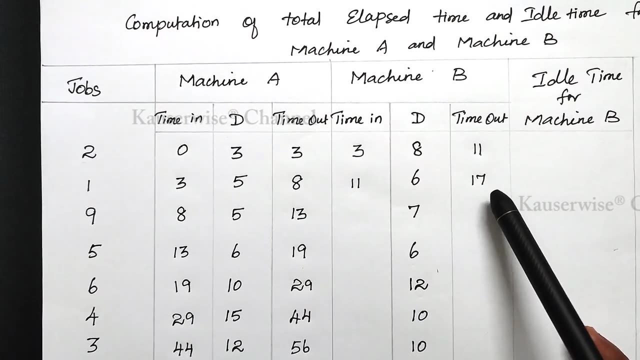 hour. So total 17th hour. So 17 is the out time for next job. okay, Look at the next job. that is job 9 and its out time from machine A is 13th hour. okay, So here the previous job completion time. 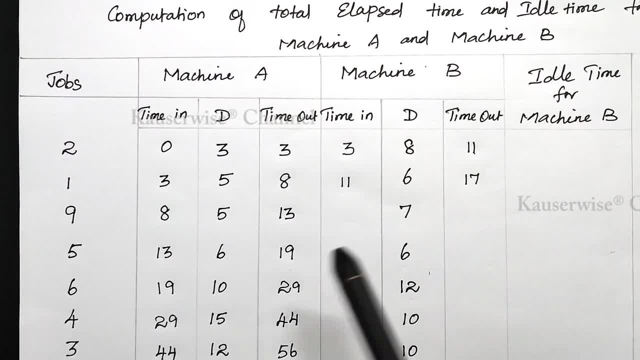 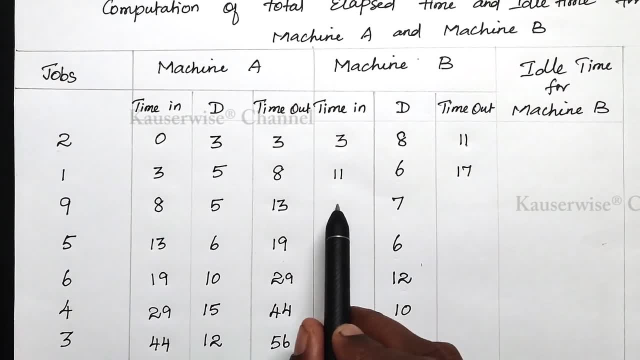 on machine B is 17.. 17 greater than machine A's current job out time: 13,. okay, So machine B can take up the next job after completing the previous job on 11th hour. So in time for the next job is. 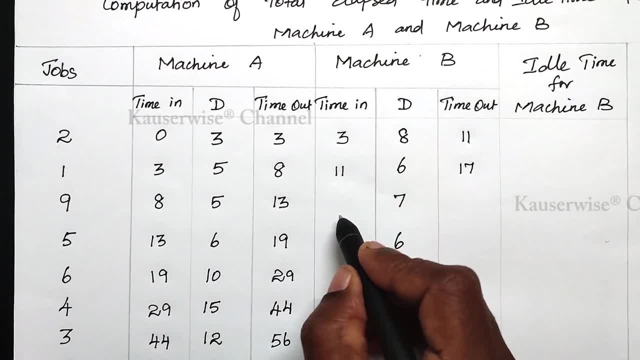 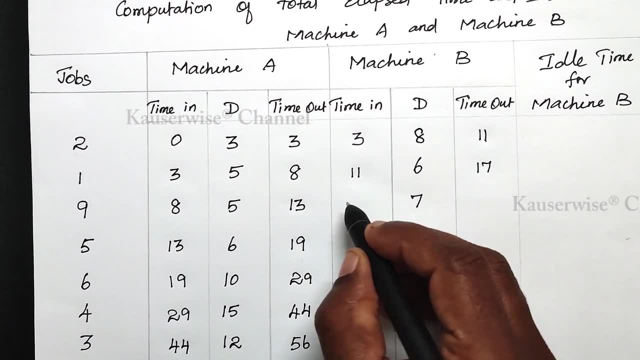 17.. So machine B can take up the next job after completing the previous job. only, right, Okay, So we need to enter greater value, that is, 17, as in time for current job on machine B. okay, So 17. 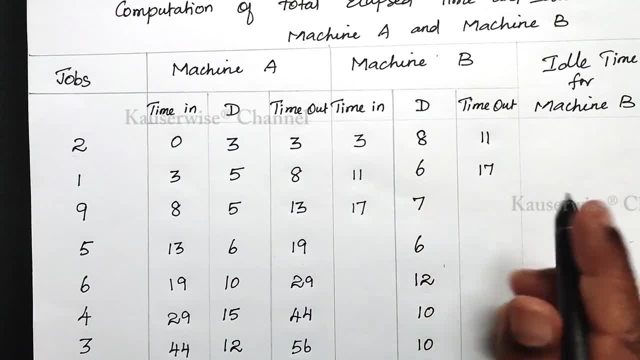 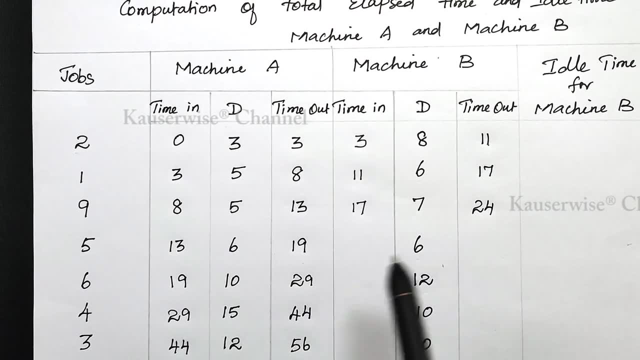 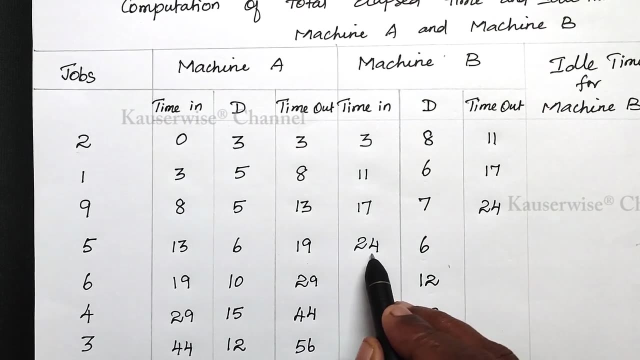 plus duration 7 is equal to 24.. So 24 is the out time. In the same way for the next job here, 24 is greater than 19.. So the in time for the next job is 24 on machine B. So 24 plus 6 is 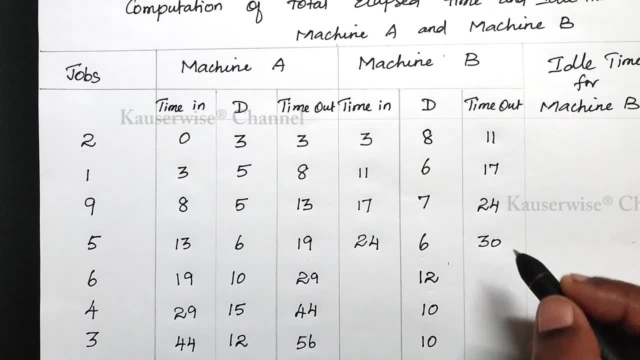 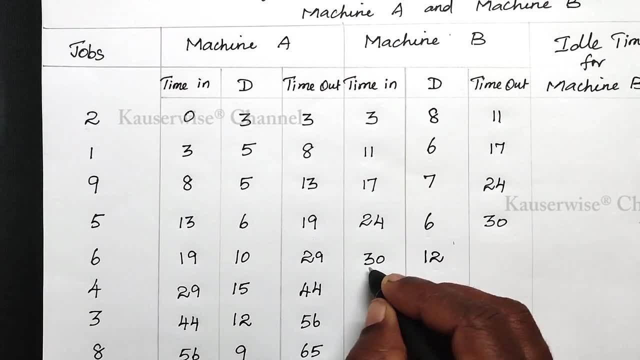 equal to 30.. 30 is the out time, okay, And the next one 30, and the next job is 29.. Now, this is the greater value. So 30 is the in time for the next job. 30 plus 12, 42,- okay, Now for the next. 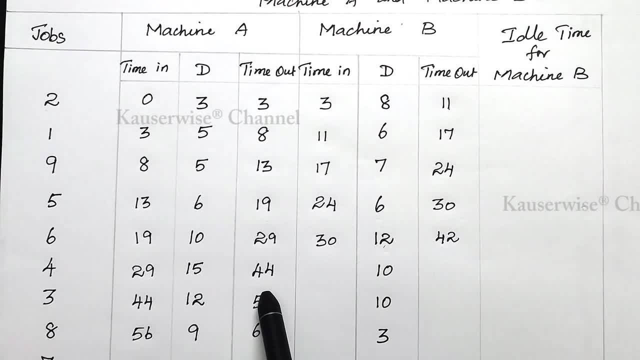 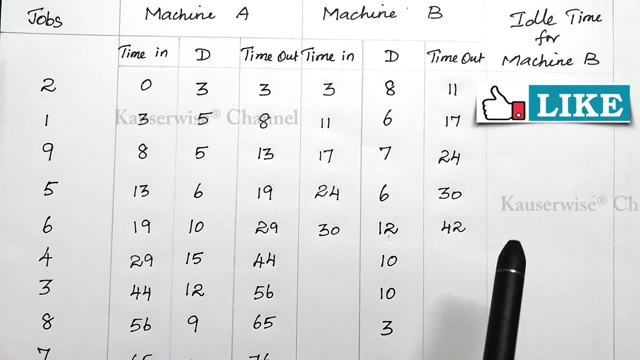 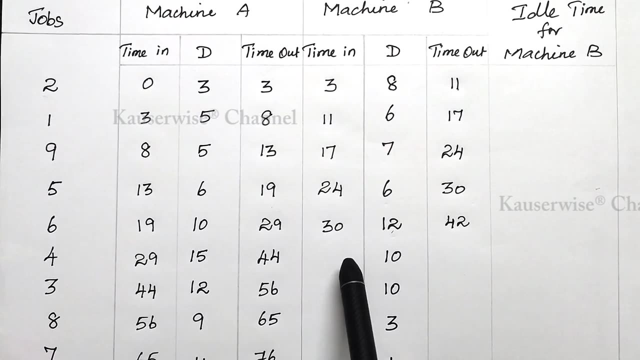 job here 42 is lesser than 44,, that is, machine B has completed the previous job on 42nd hour. okay, But the current job, that is job 4, time on machine A is 44. Now machine B has to wait for 2 hours to take up the next job. okay, So. 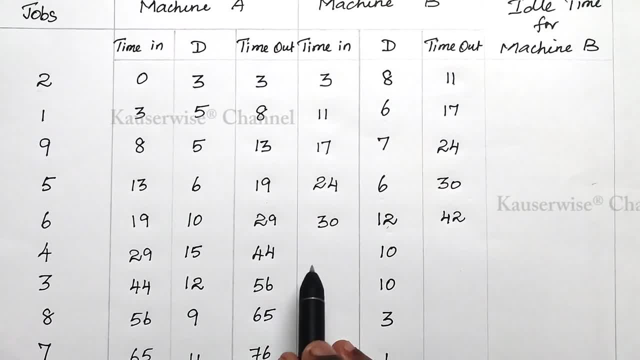 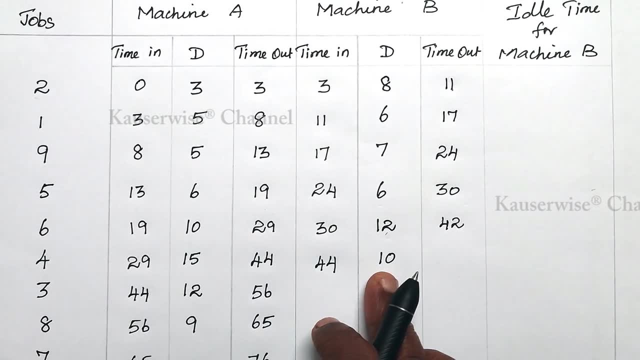 we need to put greater value as in time for the current job on machine B. okay, So 44 is the in time, So 44 plus duration 10.. So totally, 54 is the out time, okay. In the same way, 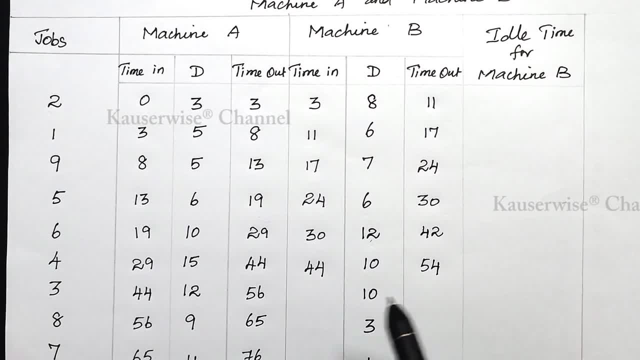 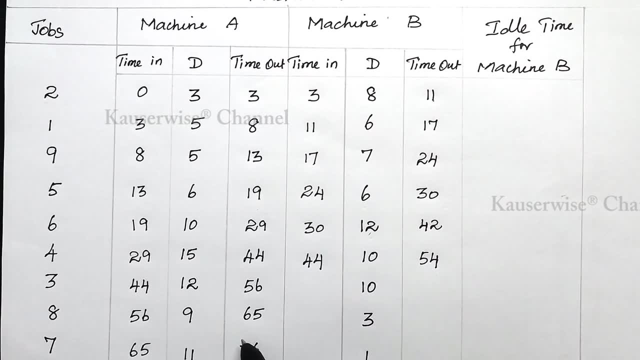 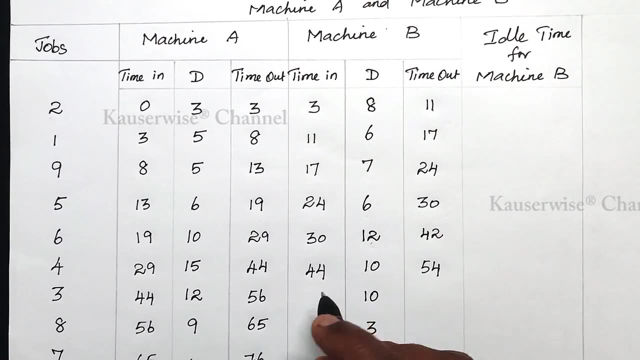 just look at the next job here 54 is lesser than 56, okay. So again machine B has to wait for 2 hours to take up the next job. okay, So we need to put greater value as in time for current job on machine B. So now 56 is the in time. okay on machine B, So 56 plus. 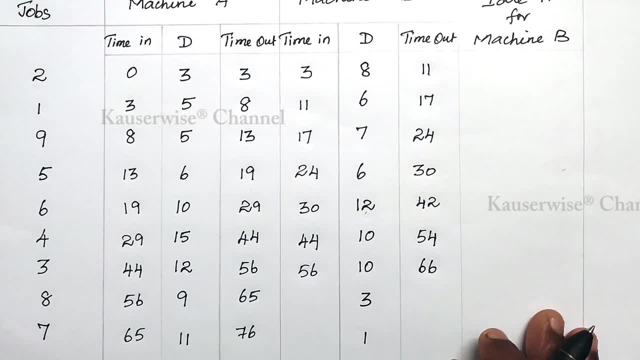 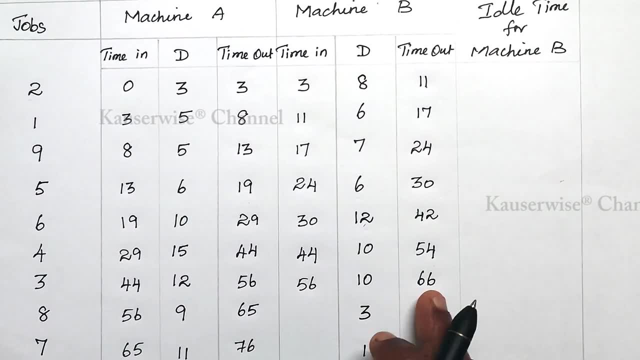 duration: 10,. 66 is the out time. okay, Now in the same way for the next one. here, 66 is greater than 65. So we have to enter only greater value. So enter 66 as in time. So we have to enter only. 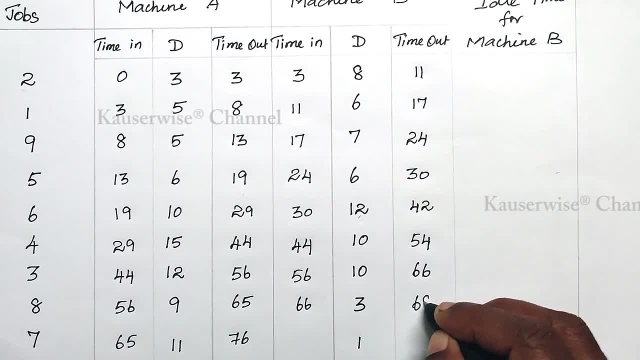 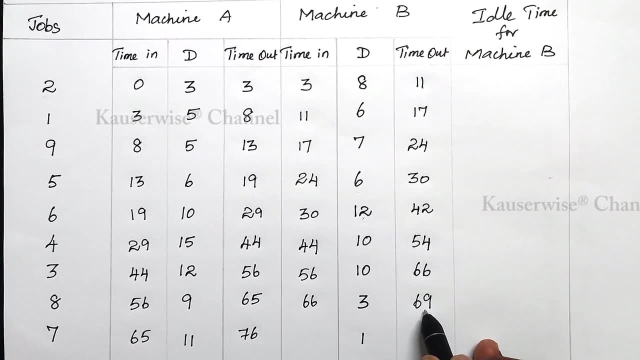 greater value. So in the same way for the next job, again we have to see the higher value. So here the out time is 69. But for the next one is 76 is greater value. okay, So enter 76 as in time. 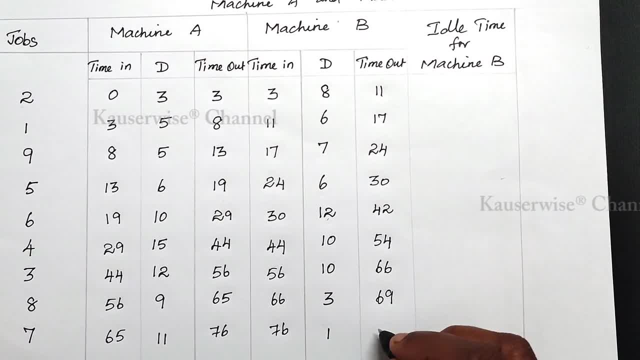 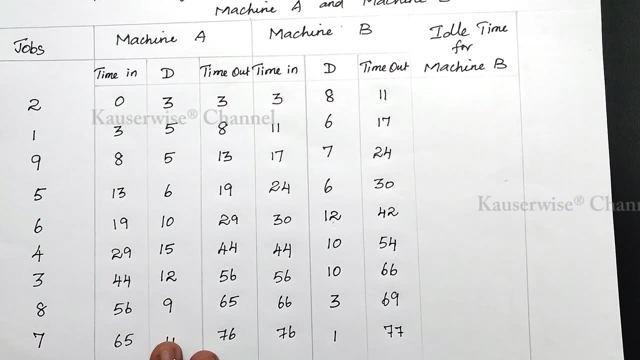 for next job. So 76 plus 1, 77 is the out time. okay, So now we have completed in time and out time for machine A and machine B for all the jobs. okay, So we have completed in time and out time. 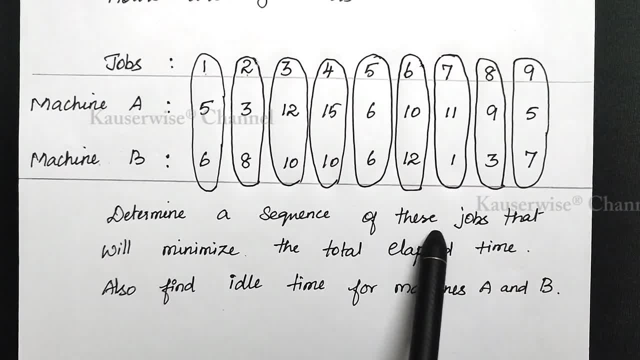 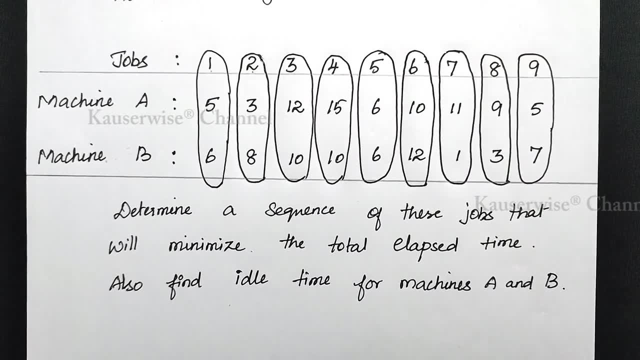 for machine A and machine B for all the jobs. okay, Look at the problem. Determine a sequence of these jobs that will minimize the total lapse time. Also, find idle time for machine A and machine B. Now let us see the calculation for finding out total lapse time and idle time for: 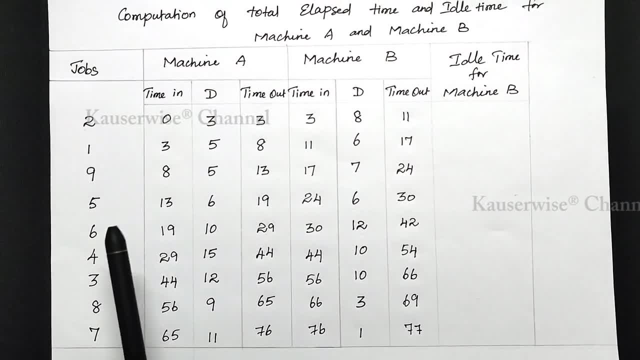 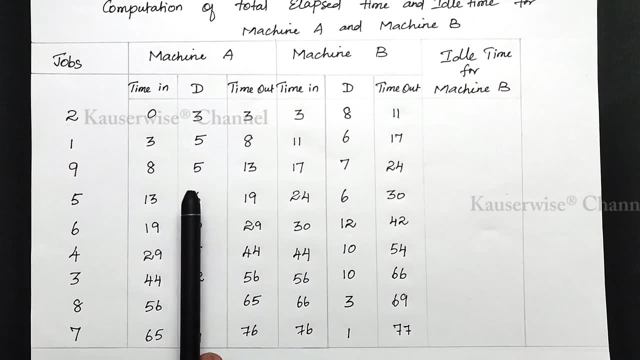 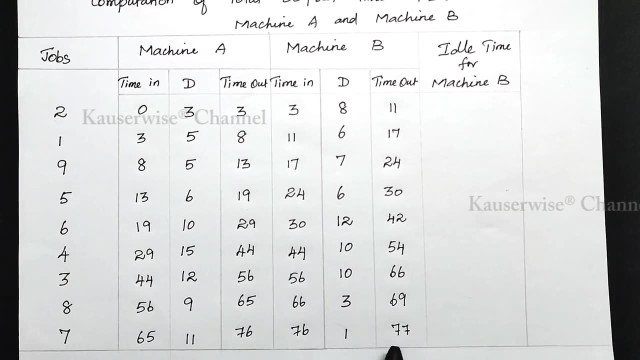 machine A and machine B: See the solution. The total minimum lapse time means the total time taken to complete all the jobs okay through machine A and machine B, including idle time. That means all the process will comes to an end at 77th hour. So this is the minimum total elapsed time. 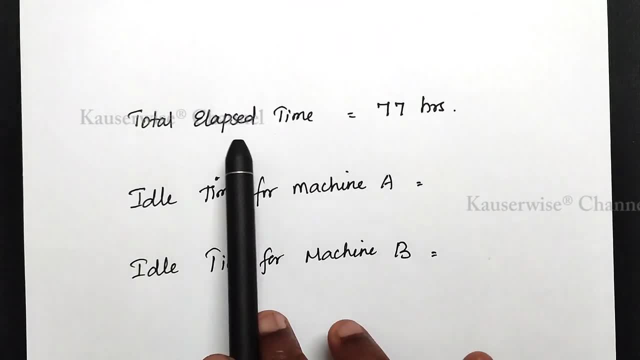 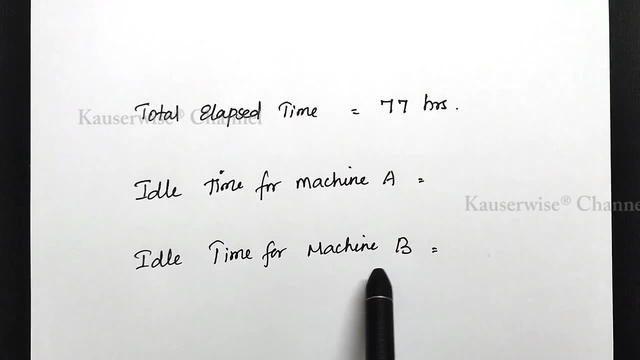 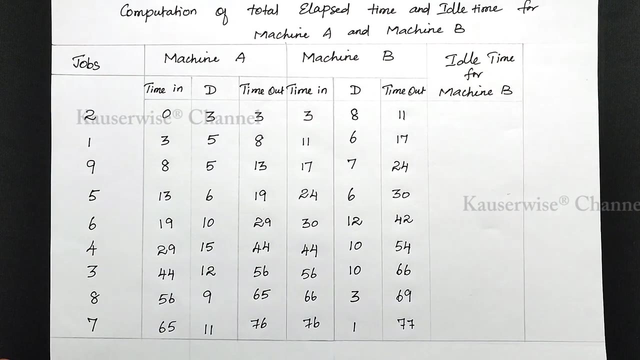 that is 77 hours. See the total elapsed time is 77 hours. okay, Now we are going to find out idle time for machine A and idle time for machine B. Now see the solution. See the solution to find out the idle time for machine A. okay For A. compare the last jobs out time. 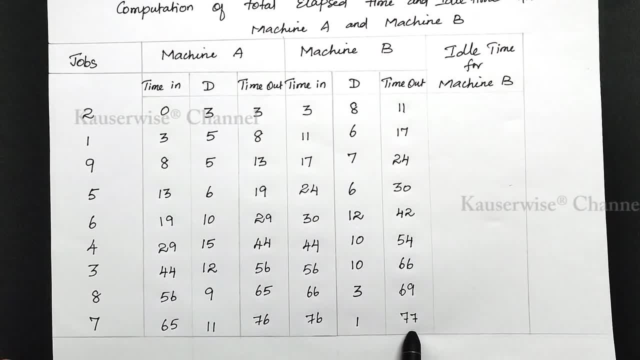 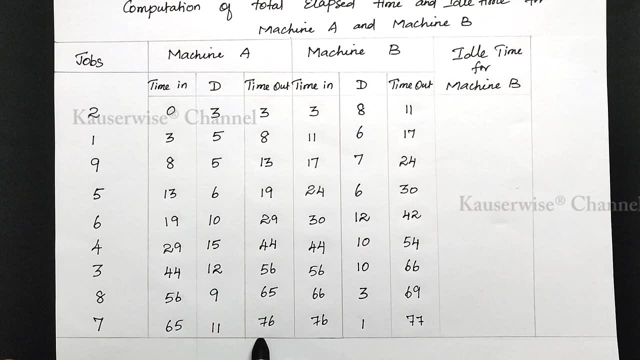 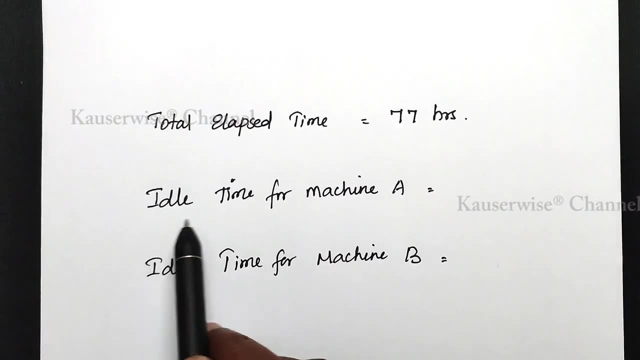 on machine A and on machine B. okay, The difference is called idle time. on machine A That is 77 and 76. What is the difference? 1. That 1 hour is the idle time for machine A, See idle time for. 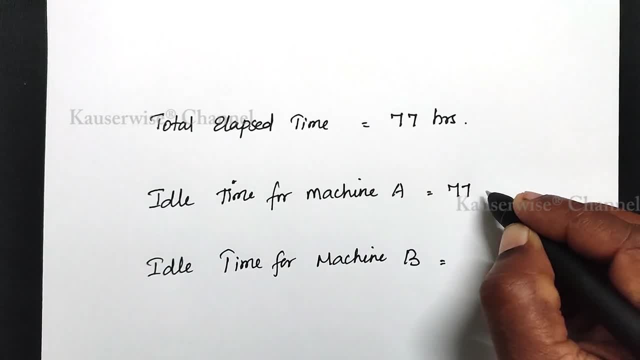 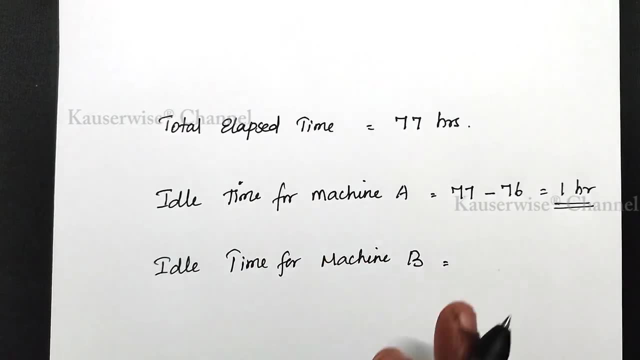 machine A is 1 hour. That is 77 hour minus 76 hour. The difference is 1 hour. So this is the idle time for machine A. Now let us see how to find out the total elapsed time for machine A. 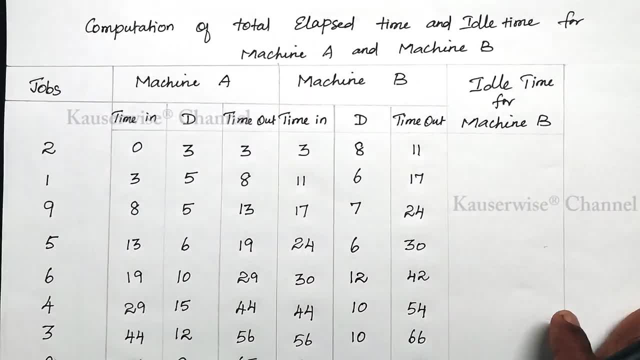 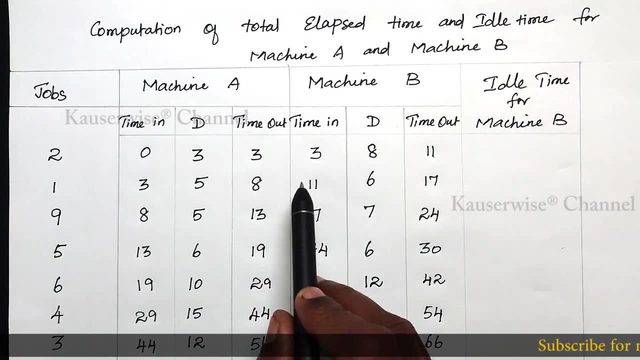 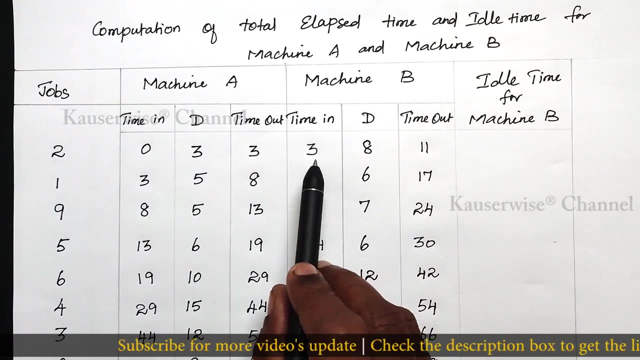 Now let us see how to find out idle time for machine B. See the solution. See the solution to find out the idle time for machine B. okay, Look at the first job here. Machine B starts its process only in the third hour, So till such time machine B is in idle state. okay, That is the idle time. 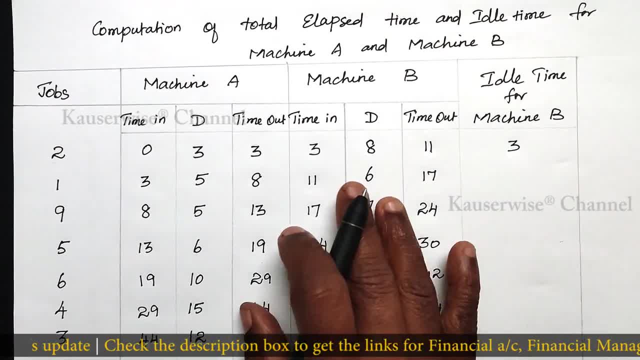 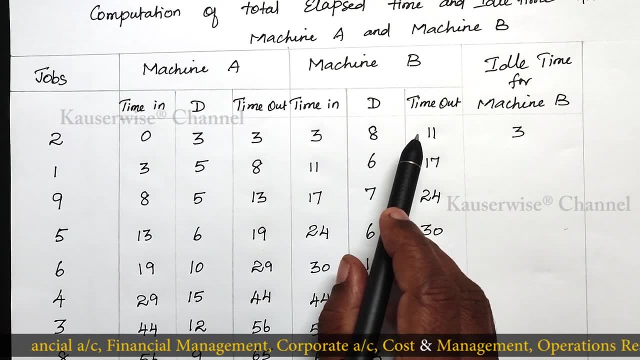 So write 3.. This is the idle time. okay, Now for the next job. we need to compare in time of current job and out time of previous job. okay, on machine B. So let us see how to find out the.